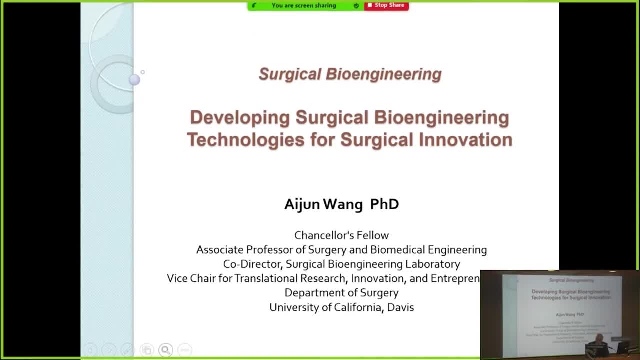 pharmacology and biochemistry and biology-related issues, Ended up in the United States in 2008 at Berkeley, where he was a post-doc fellow in the Department of Bioengineering, Kept on with that group until he joined the California Institute for Regenerative Medicine in 2010 and then subsequently came here, where he and 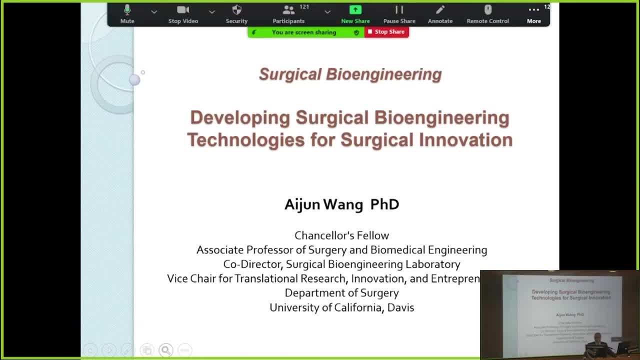 Dr Farmer, have developed the remarkable lab on tissue engineering using stem cells. in an attempt to close, spina bifida Has, remarkably, over $10 million in grants that have helped support his career and that of many others, And so I think we're very honored and pleased. 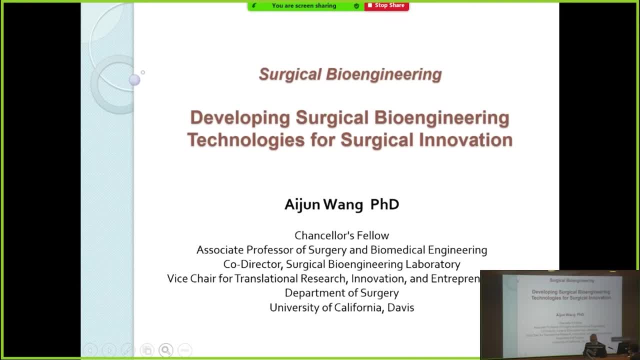 to have him and give a summary grant. Dr Farmer, I'll stay, Adrian. thank you. Good morning everybody. Good morning to the audience from the Zoom room. So it's my great pleasure to give a presentation to you all today on our research program at the Surgical 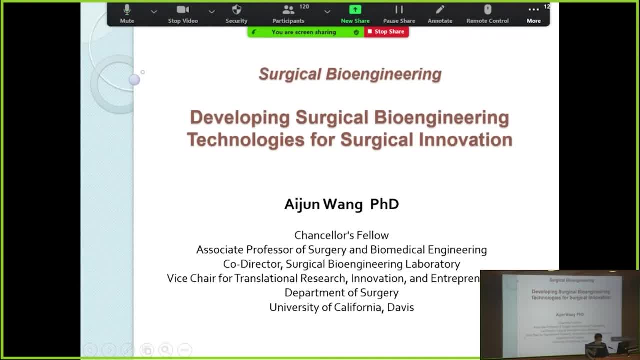 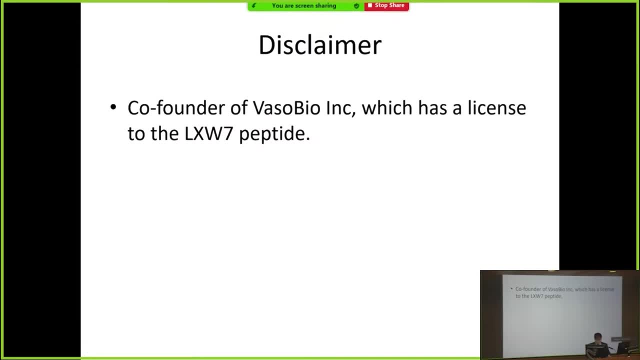 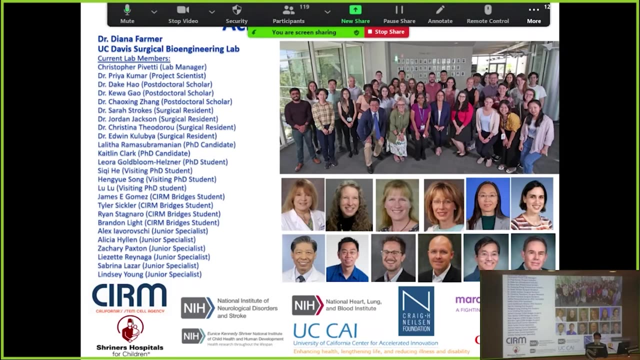 Bioengineering Lab. So I'd like to start off with a disclaimer. I'm a co-founder of VisoBio Inc. which has a license to the peptide LXW7 technology that we're going to talk about. So, before I start with anything else, I'd like to put my acknowledgments slide here, because what? 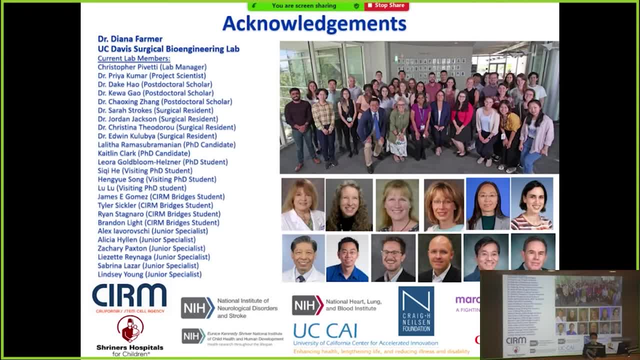 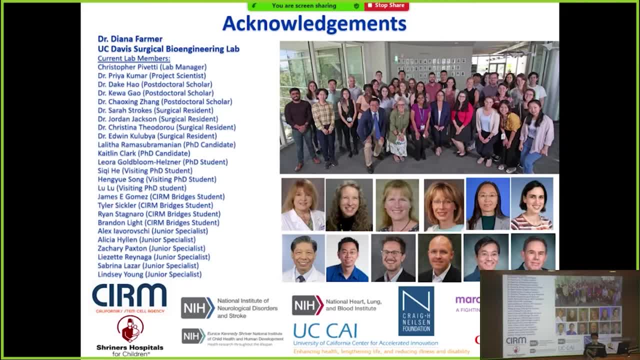 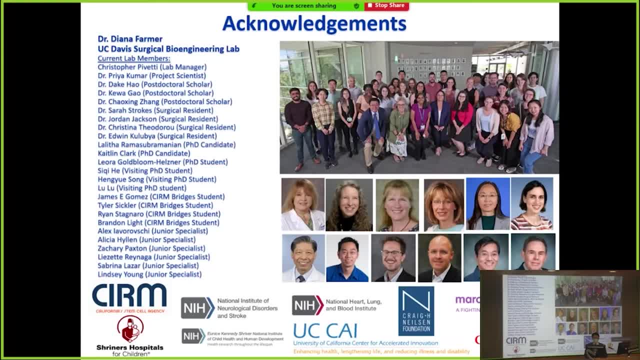 helped and collaborated with me in the lab. And in addition to our internal collaborators, I also have listed a few external, outside of a department collaborators who have made a huge contribution to our research program here, including a faculty member from our Center stem cell program from our biomedical engineering. 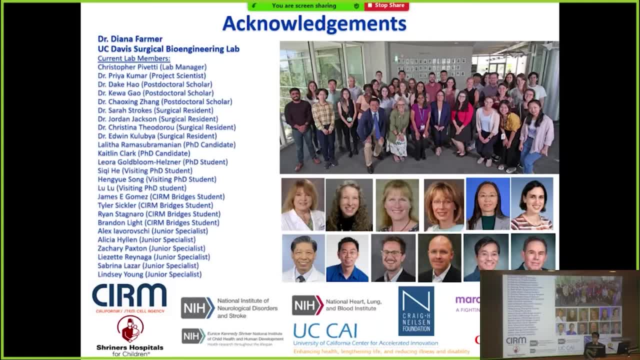 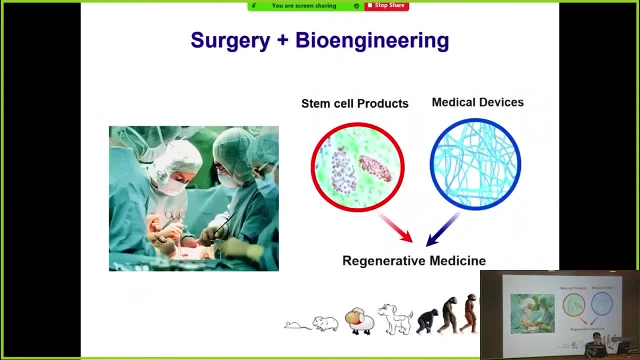 department, our vet school, our hospital for pediatric research center and also our biochemistry department at all. So my presentation, I like to give this presentation. I know now with COVID actually we are able to get probably more people who can attend to this seminar. 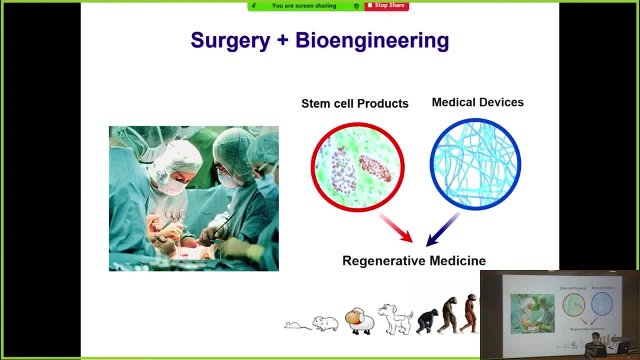 So I think I'm hoping, with this presentation, more of our trainees and also our junior faculty members and even any other faculty member who are interested in research, and get to know a little bit more about the lab at Surgical Bio Engineering Lab, what we do, what we can offer. 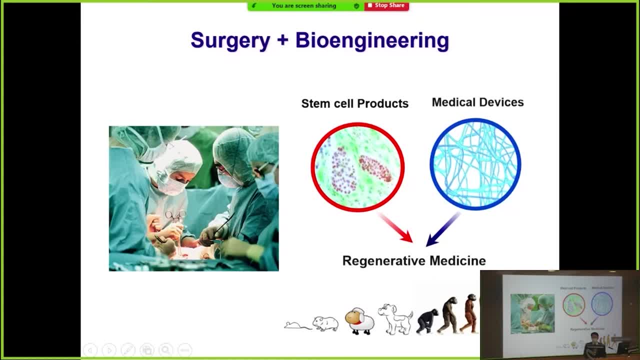 and especially for training, and see what we can really offer to the trainees, to get to know more about surgical innovation and how we can combine bioengineering, Surgical bioengineering- with surgical applications. So the overarching goal of the lab really is to bring bioengineering to surgery. 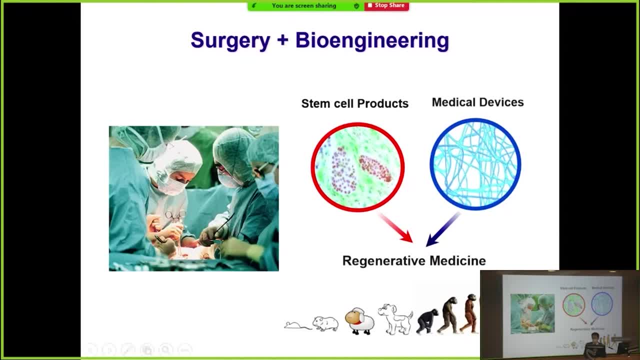 It sounds like two very irrelevant topics, But actually, as Dr Djokovic mentioned, lots of biomedical engineering or engineering at large technologies can be very well utilized to improve patient care, especially surgical innovations. So in my lab we are focused. 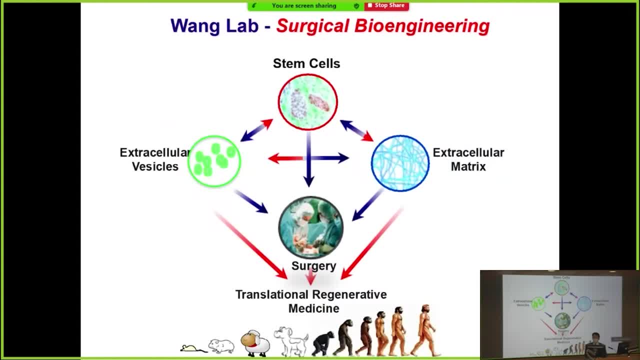 We're focused on three things and essentially you come into one thing. So we are interested in stem cells, We're interested in stem cell-derived extracellular vesicles, or we call them EVs, and also extracellular matrices, extracellular matrix molecules. 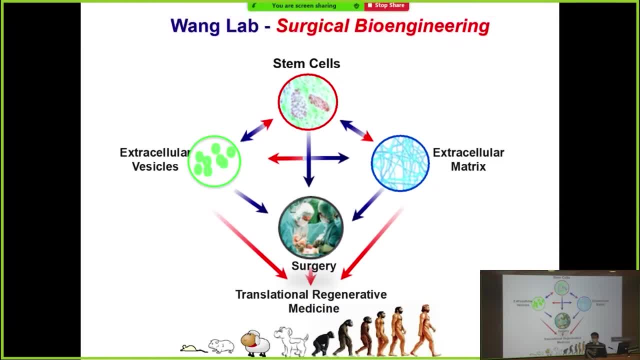 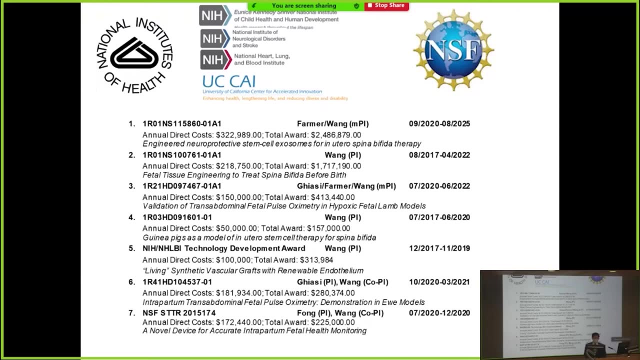 So by combining all the three or sometimes two of them together, we are hoping to develop innovative treatments for surgical conditions and diseases for translational applications. But in the past several years actually, we've been very fortunate to be funded by the federal government. 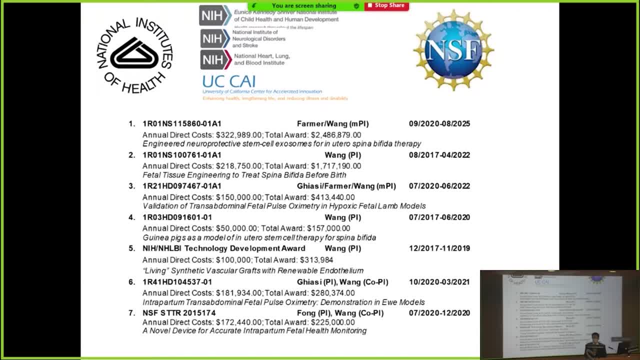 from different institutes of NIH Institute and also NSF. Currently, actually, we have two active R1s and we have R21.. We had an R3. And also we had a grant with California Innovation or UCCAI, so Center for Accelerated Innovation, I guess. 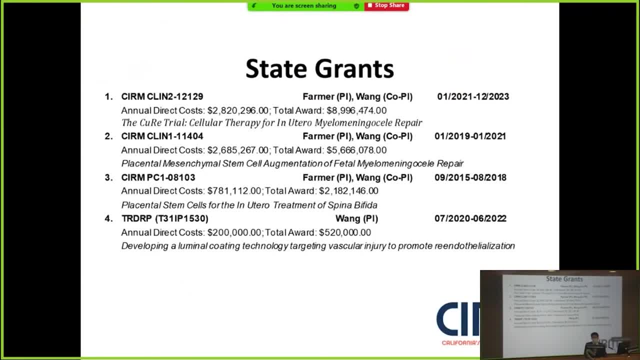 and also several other grants from NIH and NSF. So we have also been fortunate enough to get lots of funding actually from CIRM to develop our stem cell product for spina bifida, and also some other funding agencies from the state, for example TRDRP program. 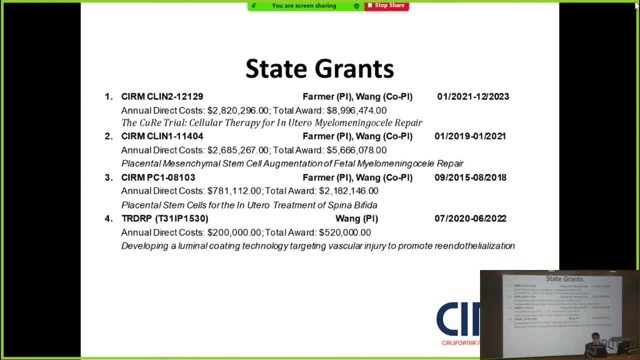 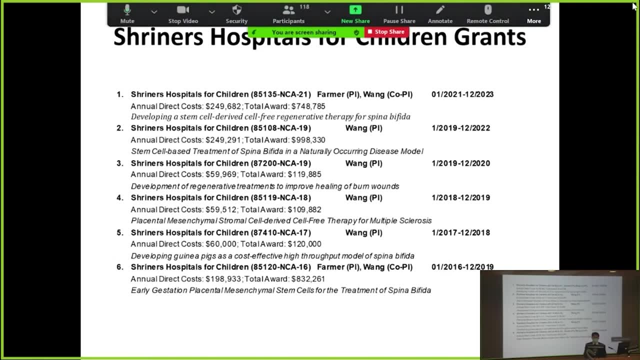 to develop technologies to treat vascular diseases. We also have received grants from Shriners Hospital. I'd like to acknowledge that too, because this has been very tremendous. It's tremendously helpful for the team to keep the focus on pediatric diseases for many of our lab. 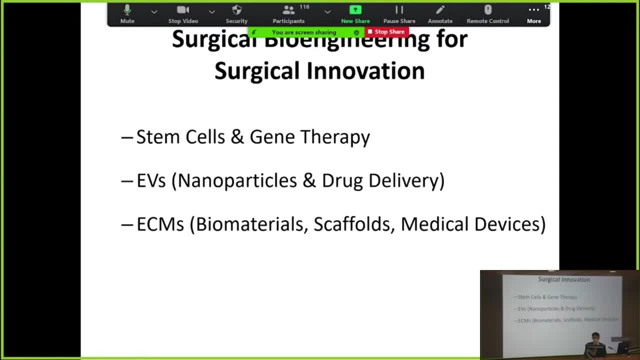 members And also so overall. actually, with all these funding support, our team has been able to develop several pretty remarkable technologies, So I'd like to highlight a few today, But if you want to know more, please visit our lab website. 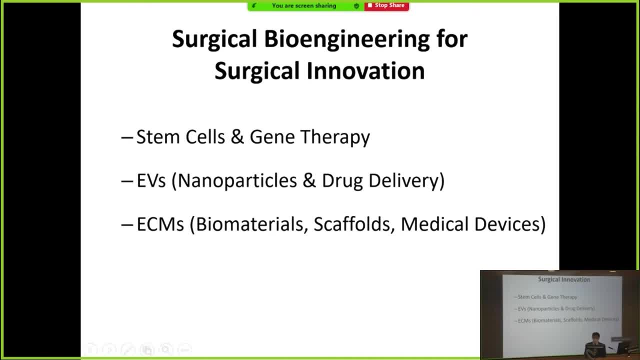 If you search my name or Surgical Bioengineering Lab at UC Davis, you're going to see more information about the lab and ongoing projects. So, as I mentioned, we have three major research directions actually in the lab. One is stem cells and gene therapy. 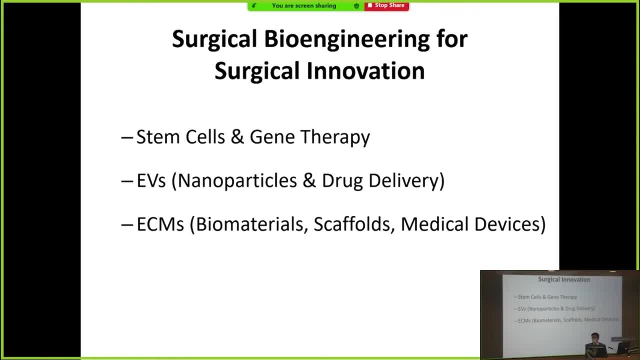 This is actually a pretty large part of the lab, But I'm not going to focus on that part. So for EVs, extracellular vesicles and ECMs, I think this is relatively new, both of these two topics. I'd like to give you a little bit of background. 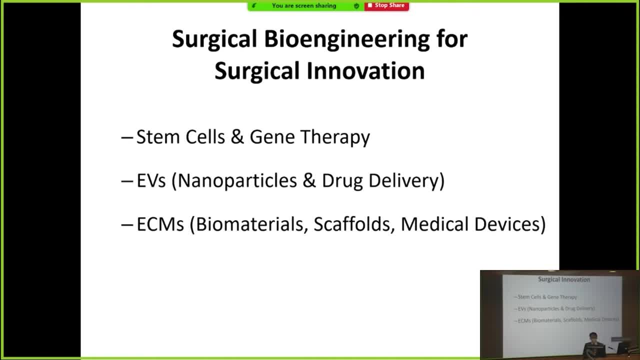 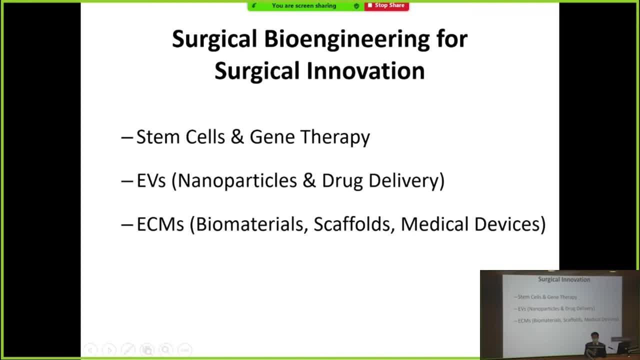 these for surgical diseases. So, for example, EVs. they are nanoparticles secreted by cells or stem cells or any cells, And they actually are a very powerful tool for drug delivery. And because they're so small, they can actually cross blobbin barrier, for example. 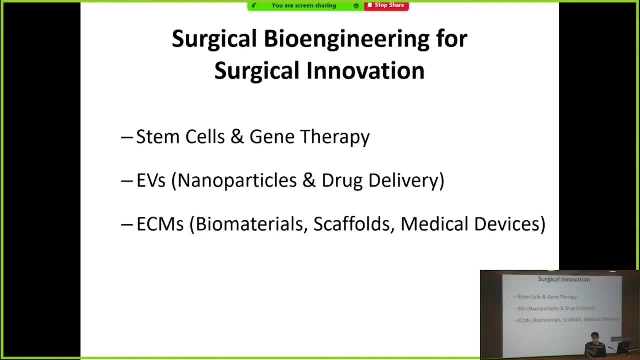 for certain applications It's quite important, And they can also be engineered. because they have membranes, they have a content inside. I'll give a little bit about that, a little bit more information later. so for extracellular matrices, actually, this is very 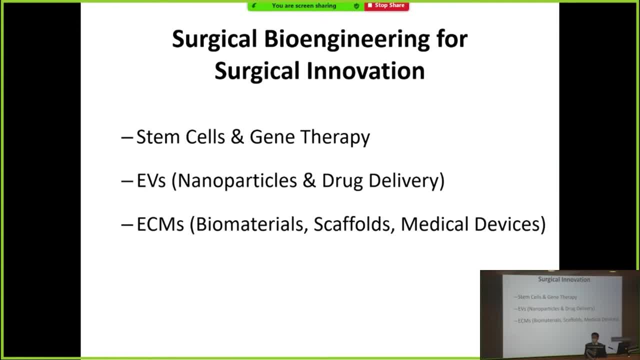 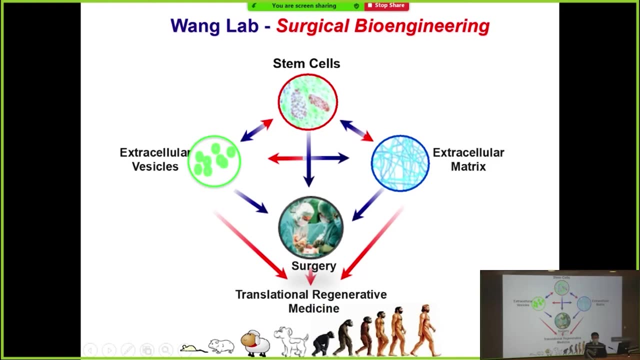 closely relevant to biomaterials, scaffold and also medical devices, because how the body and tissues and cells are interacting with the environment, the extracellular matrices are playing a huge role in modulating the interactions. so i would just very quick go through this stem cell stuff because i think you have. you must have learned, i heard about it from somewhere. 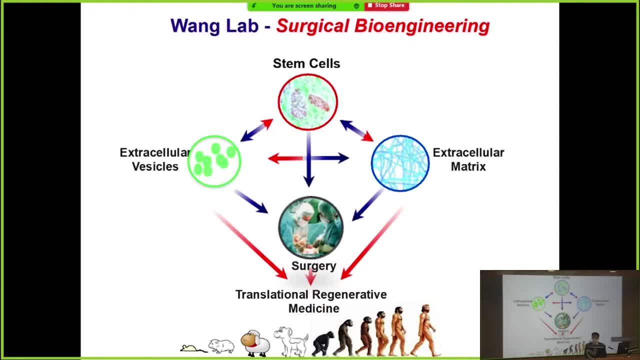 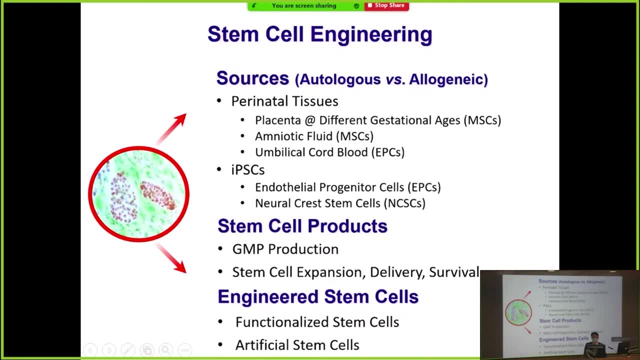 we have lots of trainees who have presented. we have faculty who are presented. i have presented before on that topic too. so, generally speaking, i just want to give you what we have in the lab, some information about that, so you you know if you need anything about stem cells. 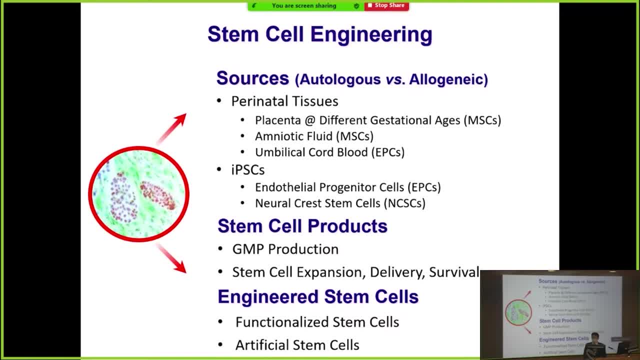 come find us. we have lots of stem cells from different sources. we also have stem cell products, for example, good manufacturing practice or gmp conco great stem cell. we have the protocol, how to do that. we have a very close collaboration with our stem cell program on campus with dr janota and gerhard bauer and their team and also we. we have a pretty 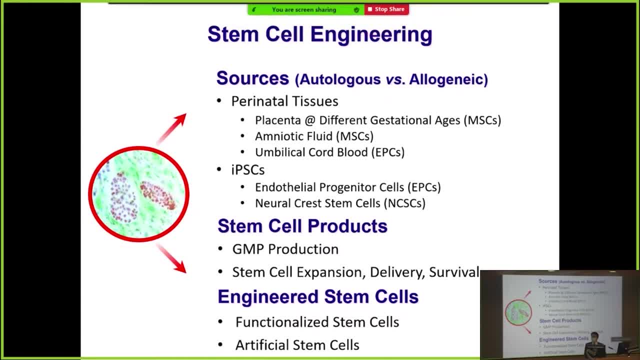 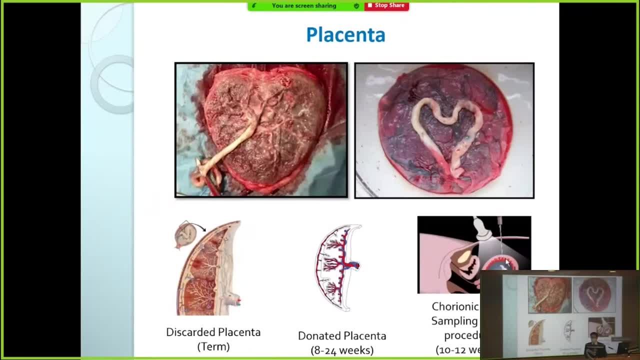 good amount of engineering work about stem cells too, how to improve the stem cell in survival or how to functionalize them. so lots of good stuff about that. one good example, though we have many others, so placenta. actually, we've been focused on placenta as a tissue source. 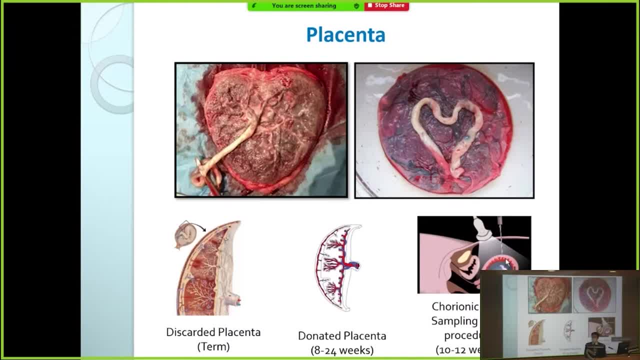 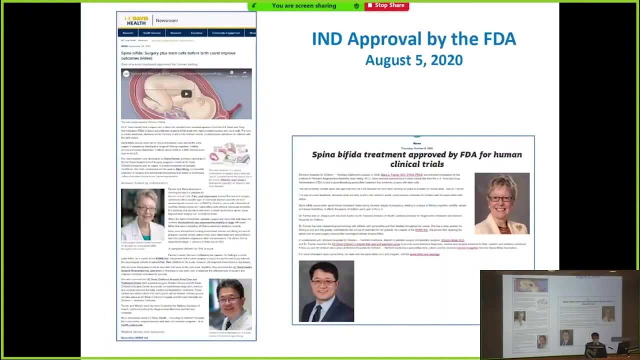 for stem cells. for a long time now we have established several different protocols to isolate stem cells from placenta tissue, even though very small biopsy of placenta, and we have identified several very unique properties of the like of these cells. so, as i mentioned earlier, we actually 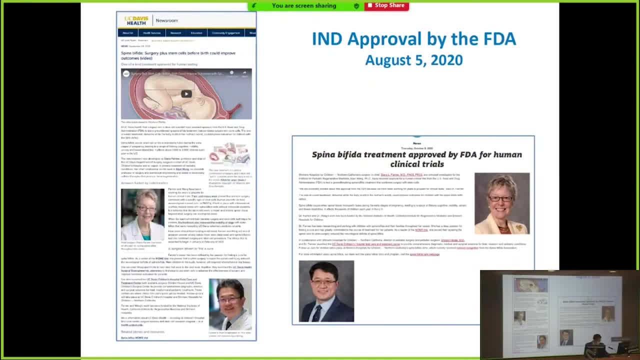 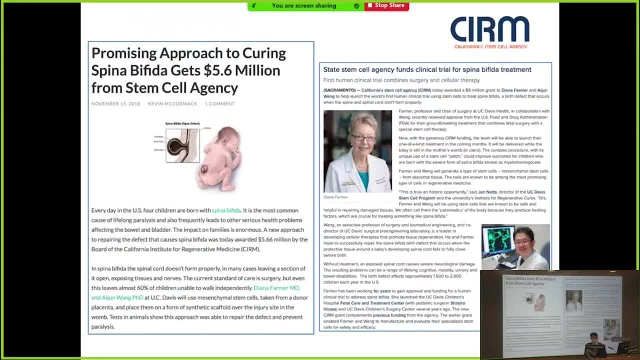 have been focused on using stem cells for the treatment of spina bifida, which has been approved by the fda. as a new ind- and actually doc- farmer and the our division of pediatric surgery team, led by dr uh shin hirose, actually are leading the clinical trial to test this new technology in the human 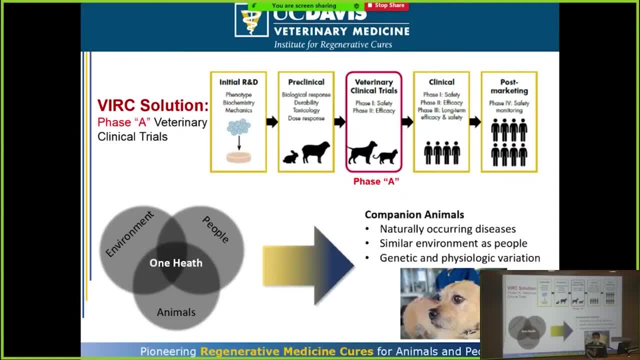 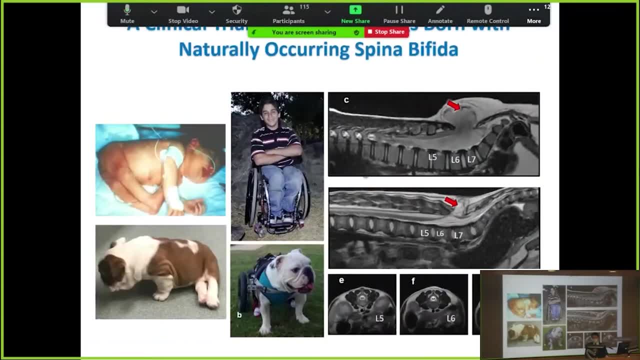 trial now. so on the same line actually, i've been leading another clinical trial from the vet school to look for a solution for a natural occurring disease model in english bulldogs. so those dogs are born with spina bifida. so they're different from the large end model that we use for research, for example the sheep model or other animal models. 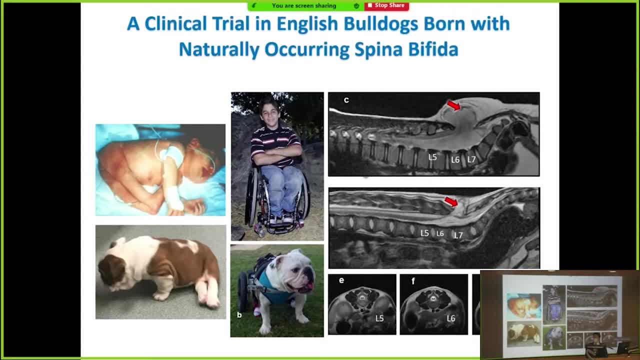 they are surgically or chemically induced. these are naturally occurring. so we actually are currently ongoing having this clinical trial, ongoing testing stem cell product for a postnatal patient- in english bulldogs. so we have made actually extremely productive year over the covet time. actually, we enrolled several patients and i can give a separate talk on that topic. 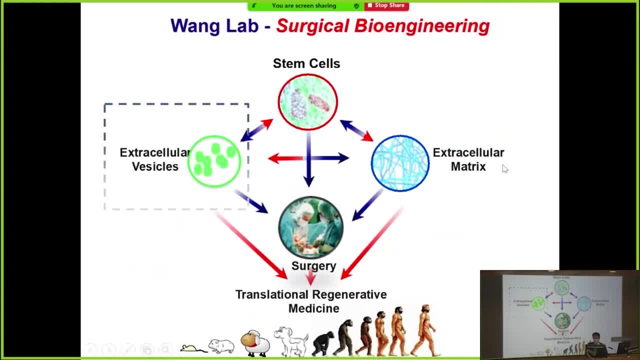 someday. so today i'm going to focus on these two things. one is extracellular vesicles, or evs for short, or ecm. i would like to give you some information about how you can potentially use these for your practice too. so evs are actually they're. 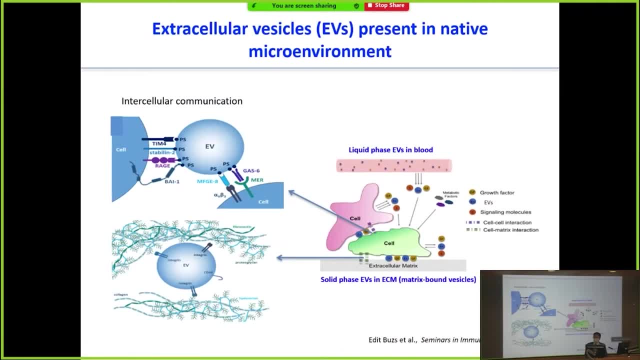 very important. they're everywhere. they're secreted by all the type of cells and they can be in either circulation as a free nanoparticles secreted by different cells, or they can be embedded in ecm, so in a tissue with the extracellular matrices. so they have 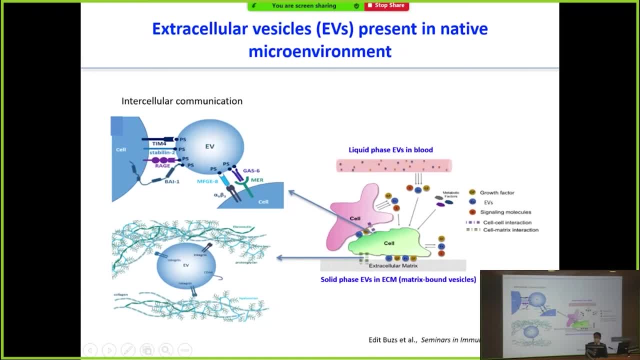 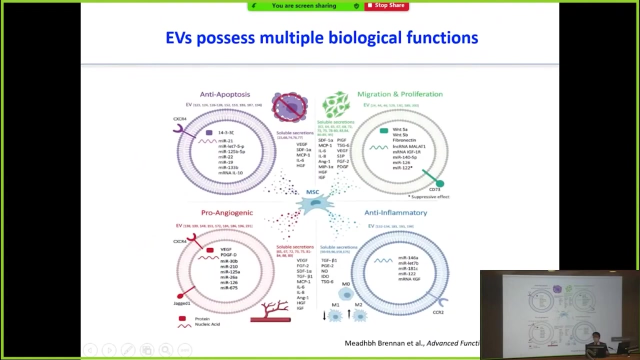 the surface, proteins on the on the other side of the nanoparticles which can interact directly with the ecm molecules, for example collagen. they also have lots of good stuff inside cargos of nuclear acids and proteins, especially micro rnas, which are really interesting to our research program. so we're trying to actually understand first of all the biology of the, the evs and 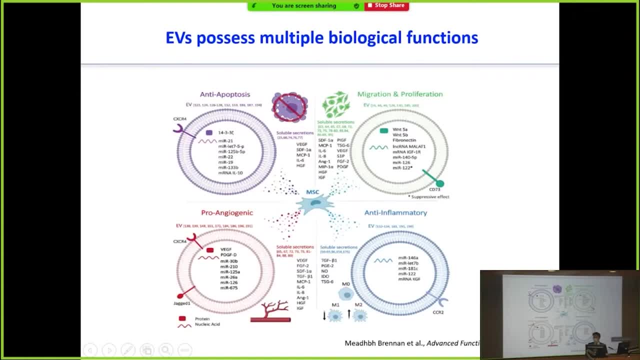 especially the therapeutic potential of these evs. for example, we know evs are having uh potentials for anti-apoptosis, migration and proliferation of the recipient cells and also pro-angiogenic functions and also anti-inflammatory functions too. so they're very versatile, they're very multi-functional. 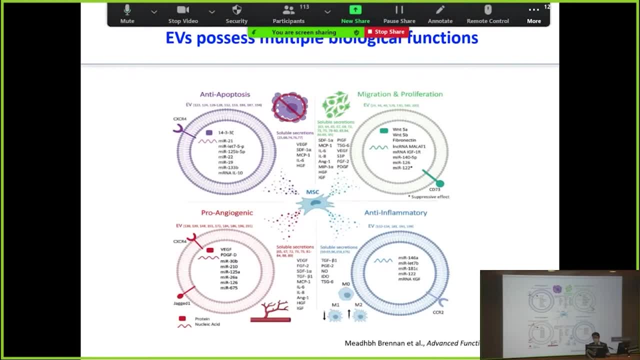 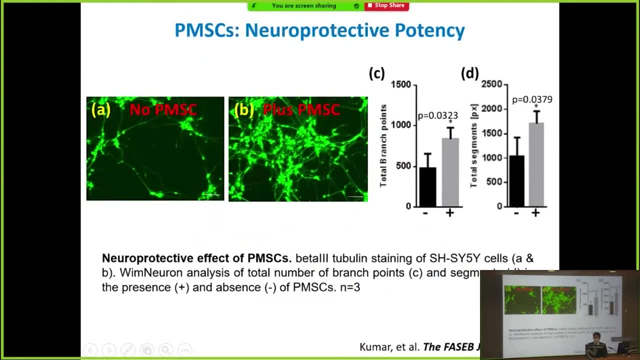 but how to use them very like effectively and establish them as a therapy is something we're really interested in. so in our own research, actually the past several years, we found that if i, if i give the talk about the stem cells for spina bifida, i would have to give you a video. 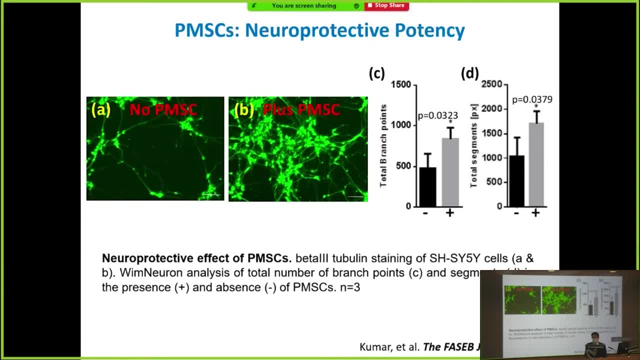 showing that with our stem cells, actually the lambs with spina bifida were able to stand up and walk with the stem cell treatment, compared with the control without stem cells. the lambs were not able to stand up and walk, and we later find out, actually the stem cells are mediating neuroprotective. 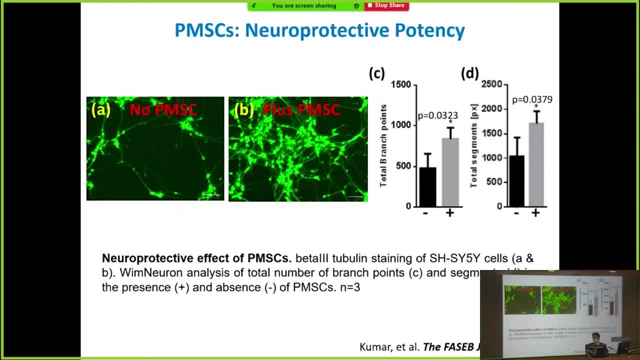 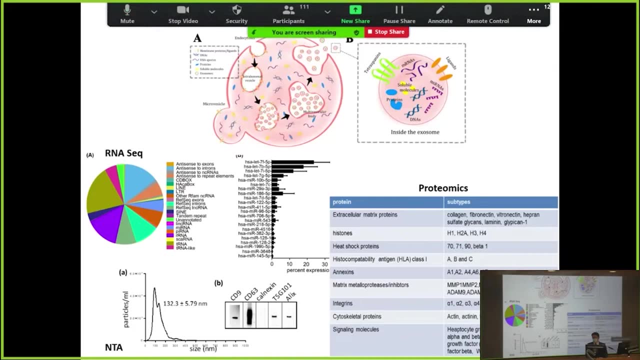 functions, so the stem cells can protect neurons. now we have the model in the dish showing that m pmsc's or placenta mscs are able to rescue neurons from apoptosis. we're also seeing this in small animal models too, but we're also seeing that pmsc's and or msc's at large 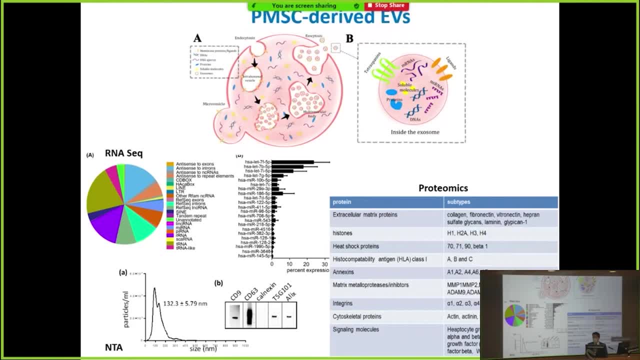 that after transplantation, they don't necessarily stay or stick around for a long time, but the effects or the function outcome actually tend to stay long. so how? how is this happening? what's going on with this? we actually now is more, we're more focusing in this area, which which is called msc secretome, so which means the cells are secreting. 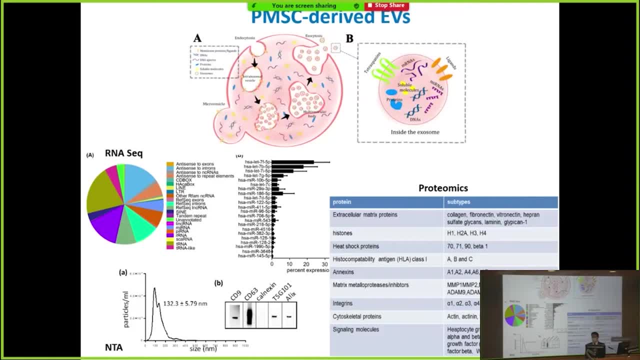 lots of good stuff to the environment that can be carried forward even without the cells being there. the stuff is such as, excuse me, extra cell vesicles and other proteins and cytokines- they can actually be around for a long time- and especially evs. so this is why we actually start look, looking into 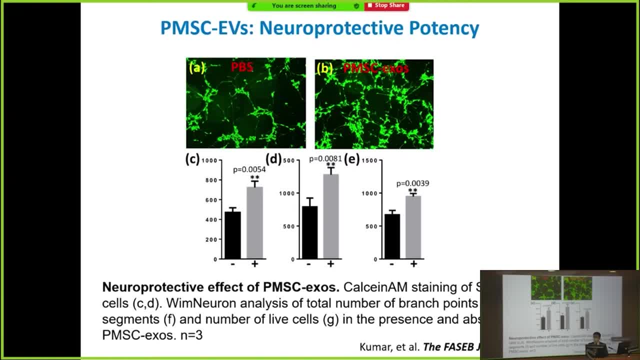 the application of evs. by using evs only, basically, you collect the condition media, isolate the nanoparticles from the culture media, actually without using live cells, you can see that they- this is the control, without using evs and this is a cells neurons- in in apoptosis with evs, you actually act, or exosomes in this case. you can see that with the ev treatment. 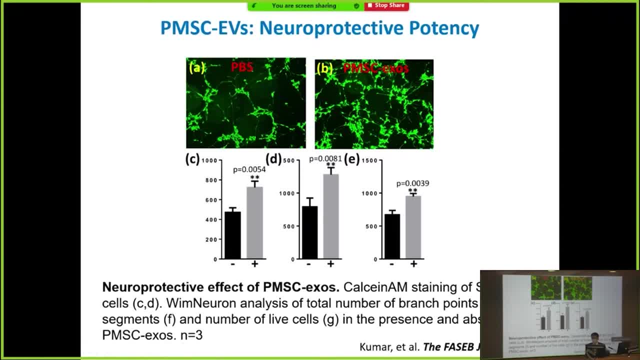 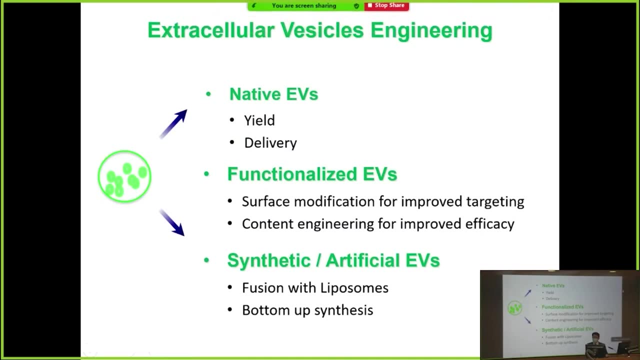 more neurons can be protected. this indicates that you probably don't need to use mscs in some cases, and just using the msc derived evs could have some neuroprotective functions. and then the key question now is that with several other animal models actually ongoing, 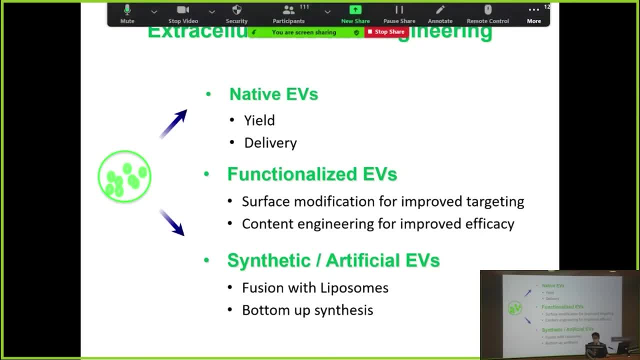 right now that we we are asking a very critical question for development of the technology for clinical use: how to get this enough and how to get this treatment more effective. so that's why we're actually interested in looking into how to get the cell culture condition to be. 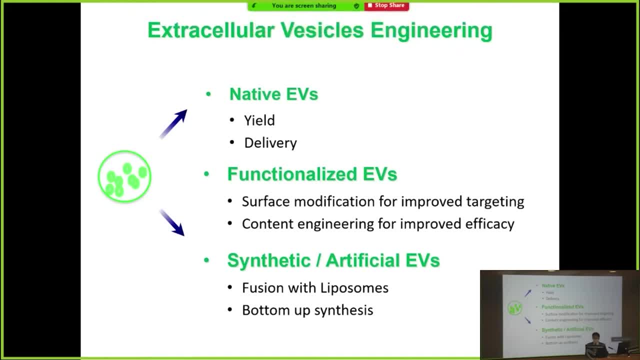 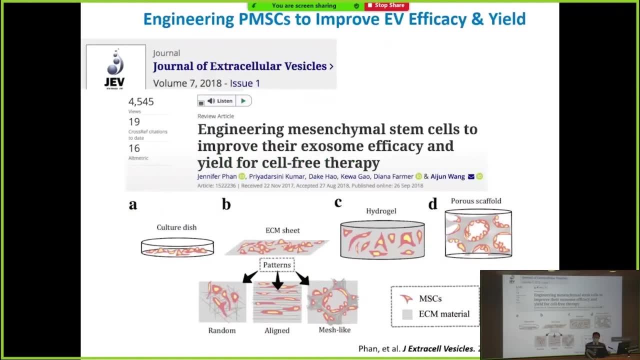 more, be able to provide a higher yield and a larger quantity of evs, and also how to functionalize evs and make them more effective in treatment. so this is one example that we've been looking into using different extracellular environments, including 3d biomaterial scaffolds or bioreactors. 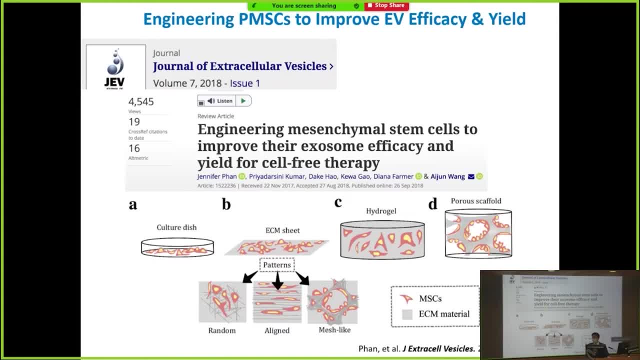 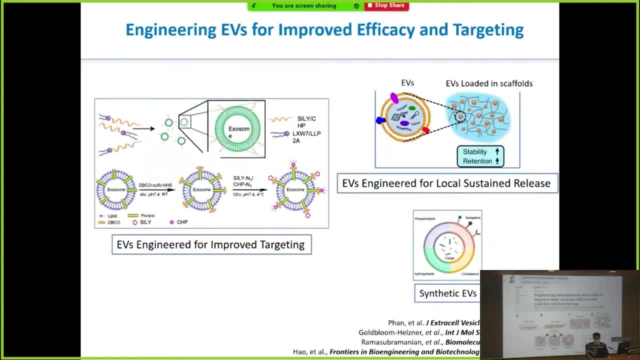 to look for ways of expanding the cells so that we can have enough evs, and also looking for ways to control the quality of evs. so there'll be. they are more homogeneous rather than heterogeneous, so, which is a very important part of the product development down the road. so we're also very 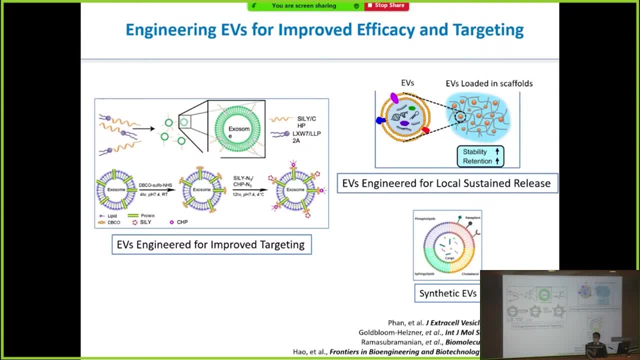 interested in engineering evs to be targeting and also to improve their functional therapeutic efficacy. so, for example, you can actually imagine there are small cells, even though they're not live cells. they're small nanoparticles. you can engineer the surface with different ligands to target disease area or specific type of cells. you can also engineer a scaffold to load extracellular vesicles. 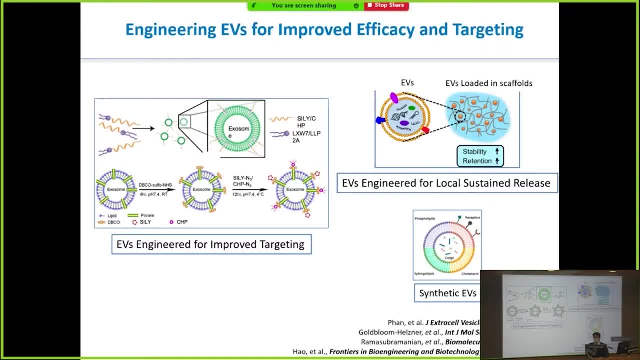 or biomaterial or hydrogel to load extracellular vesicles, to local delivery, for a sustained delivery as well. ultimately, actually, you can actually synthesize evs from scratch, from bottom up, using bottom up, bottom up, scratch approach to make your own evs as you like, as you can imagine, you can. 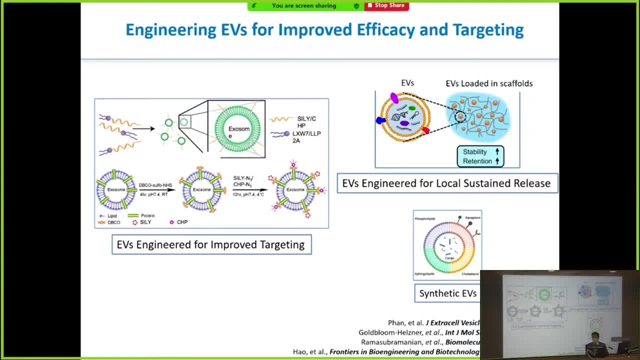 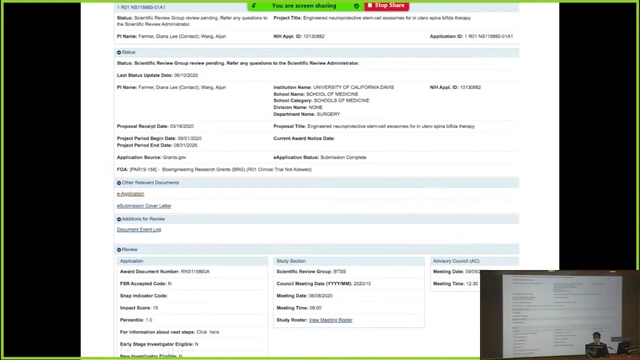 actually use different technologies to modify evs for different applications. we have a lot to do and we are having quite a few different projects about ev engineering right now. so this is one example, which i'm not going to talk about other applications today, but i think at one time i will tell you more about how ev engineering has. 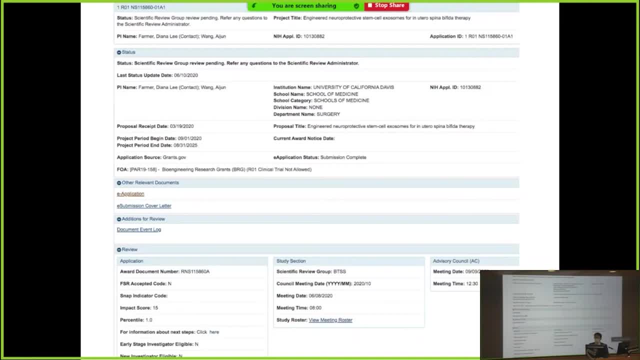 been done in our lab for different disease applications. we apply for new r1 to the nh. actually by using the ev delivery system for derivation into some methods. the common relationship between a new device we cannot ط. let's see the colon. we use the accompiro on此 criteria. acrochromyca وه p beni. 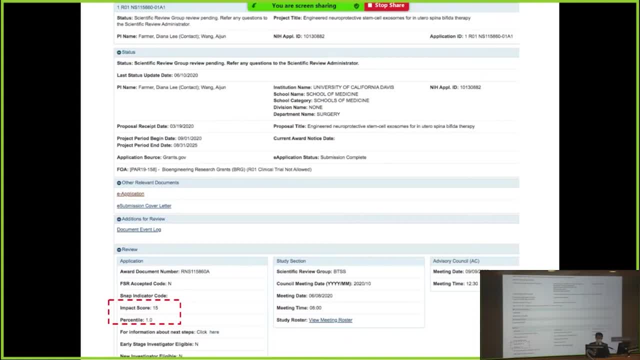 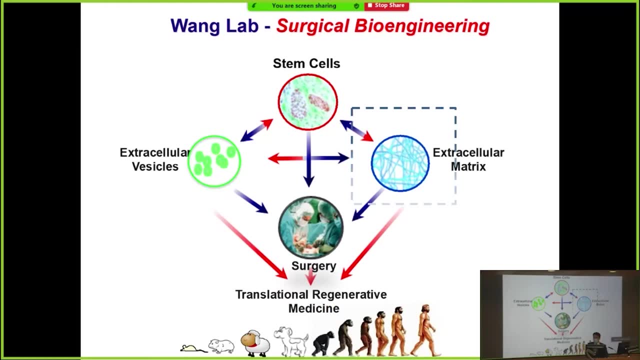 and to develop some possible strategies to detect exposure of a 때는 mo조 and clear. i'm sorry, i thought i would plug in this example: how, how, p, how, how, how, how. I think I'm doing good now We have time. So extracellular matrix actually is even also very important. 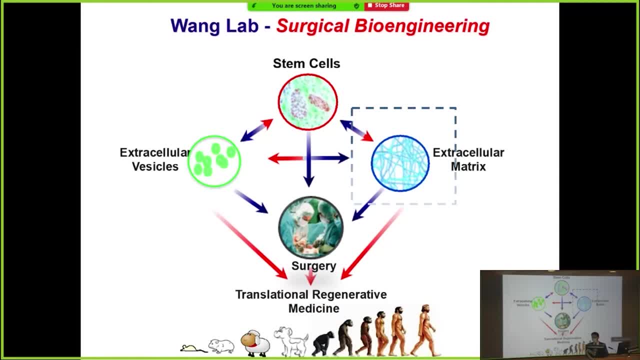 and interesting because this is closely relevant to medical devices that all our surgeons are dealing with almost on a daily basis. Because the cells- when you have a medical device implanted in vivo, the body and the cells will interfere directly with the medical device. 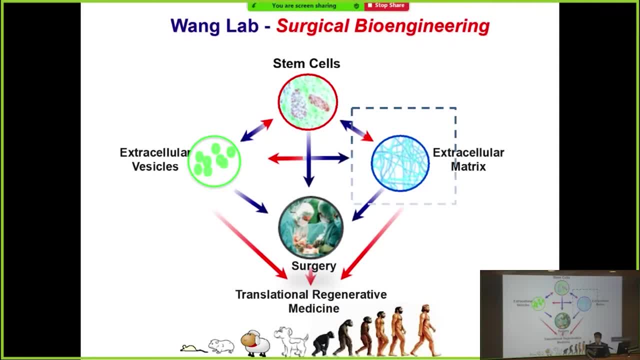 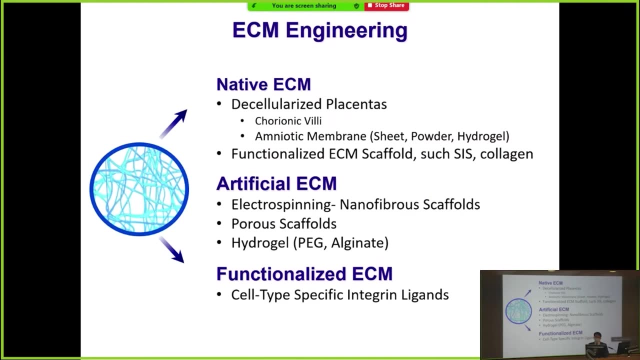 And how the medical device is interacting with the body actually is something that we can learn from the native environment- how the ECM molecules are interacting with the body cells. So we're learning this from several different ways And also we're trying to develop ECM technologies. 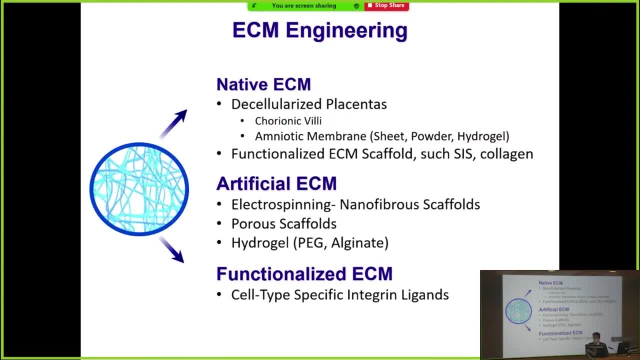 into surgical technologies and products. So we're interested in native ECMs. Basically you can derive ECM from different tissue, from human or from animal tissues. by decellularizing, by functionalizing those ECM scaffold, make them into scaffold. There are several very successful clinical products. 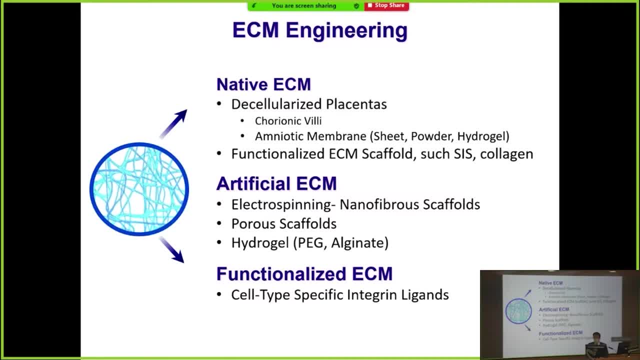 For example, small intestinal submucosa or other collagen products that are widely used in clinic scenario. actually, We are also interested in deriving ECM materials from different tissues for specific applications. I'm not going to focus on that. So we also have these two technologies, which 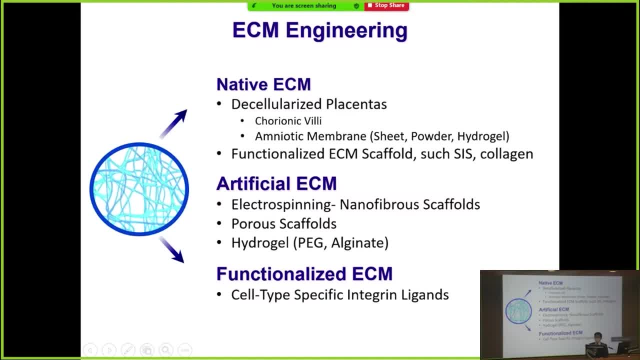 one is artificial ECM. So how to make the ECM to be more tissue function specific? This is something we can do by using bioengineering technologies. For example, you can use electrospinning technology to make nanofiber scaffold which is similar to the native. 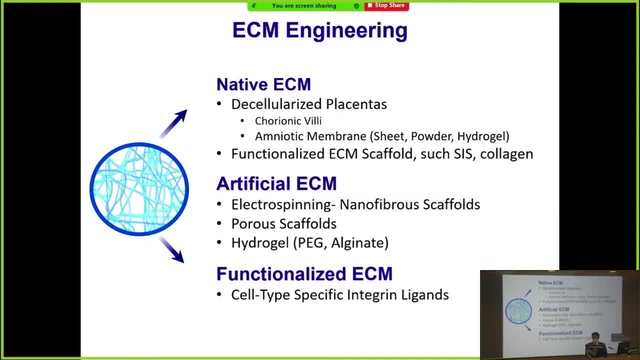 ECM nanofibers And you can also add different ligands to functionalize ECM, to mediate specific cell ECM interactions, basically to modulate the recipient cell functions, for example by modulating binding and also downstream signal pathways, by having a specific molecule on your medical device surface. 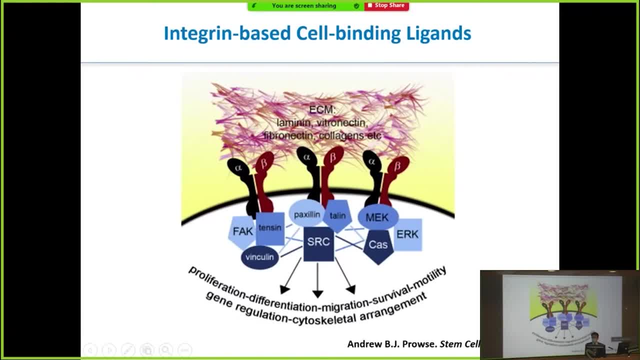 So one example of the regulating pathways for cell or tissue functions is the integrin-based ligands or integrin-based pathways. So integrins are playing a huge role in mediating cell-cell interaction and also cell matrix interaction. So that's why we're interested in that. 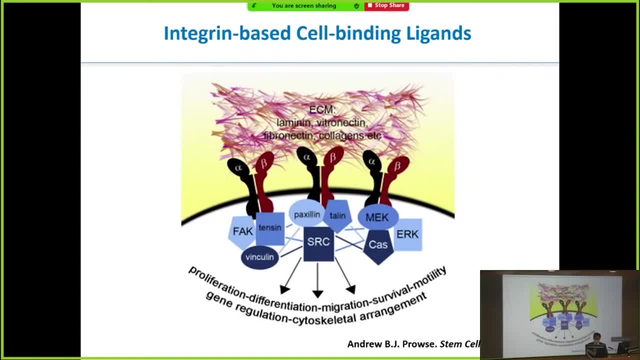 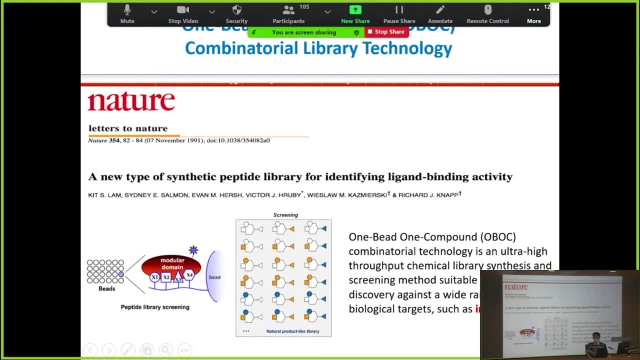 And also at different stages and different type of cells, they have different integrin molecules. So by using a one-beam, one-compound, high-throughput screening system and collaborating with Dr Kit Lam from biochemistry on campus here at UC Davis, we actually have been 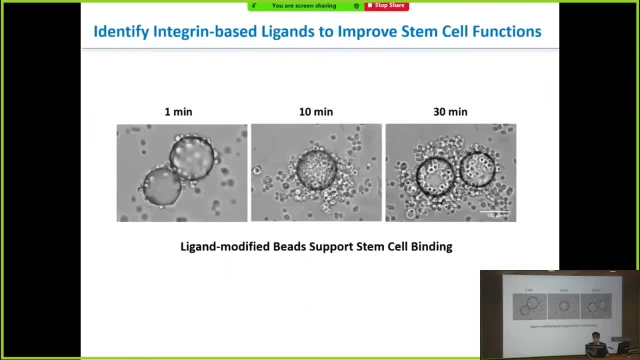 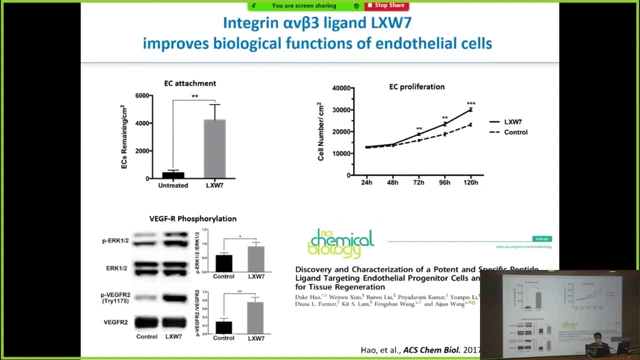 able to identify several ligands using this high-throughput screening system to target specific stem cells, For example. we have very much interest in endothelial cells because endothelial cells are so important in vasculature, in everything about healing and regeneration. We identified a ligand. 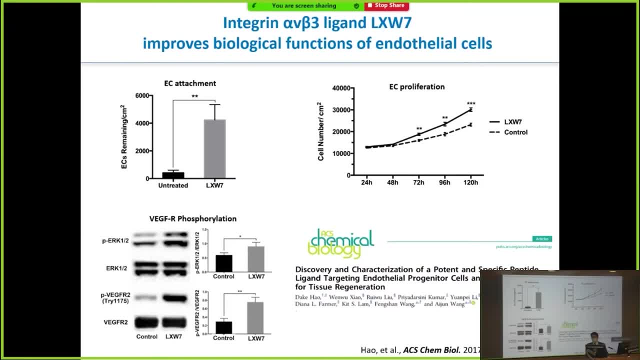 I think I presented this previously. This ligand actually so far has been shown very, very potent in modulating endothelial cell binding and also the endothelial cell surface receptor, VEGF receptor phosphorylation, which is a huge deal for the function. 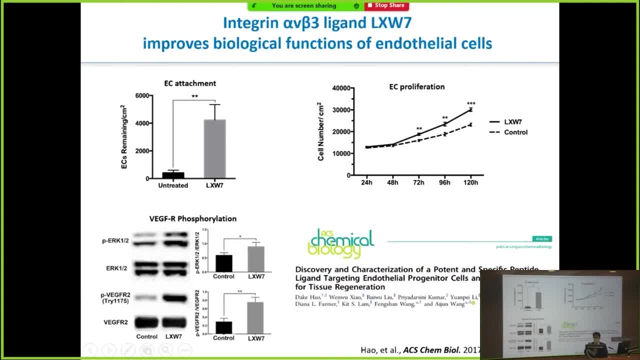 of endothelial cells And also endothelial cell proliferating, which is a huge deal for the function of endothelial cell binding and proliferation. So basically, you can imagine having this ligand on a surface, that endothelial cells either being recruited from the body. 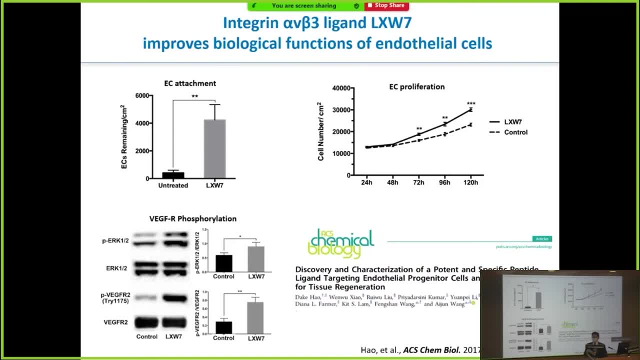 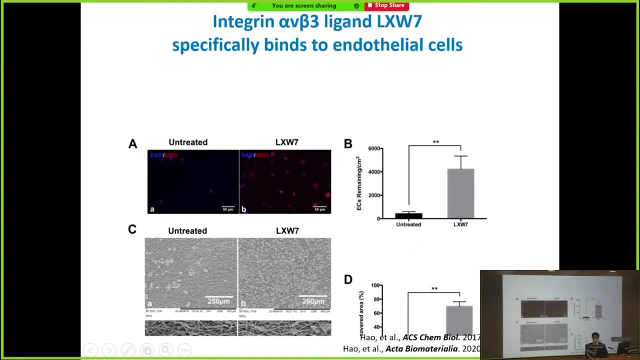 to the medical device surface or being transplanted by co-culture cells on the device ex vivo and then transplanted vivo. You can actually imagine the cells will be in a different status now with the exposure to this ligand, And we actually have shown that by having this ligand. 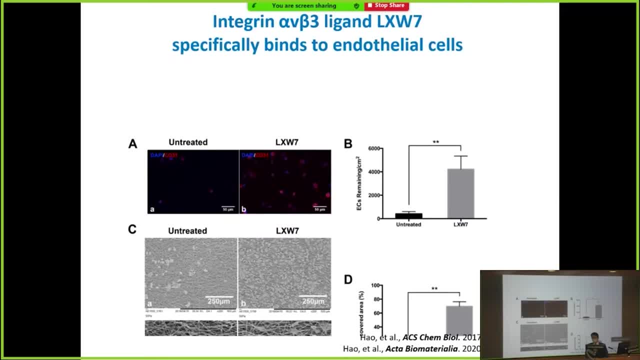 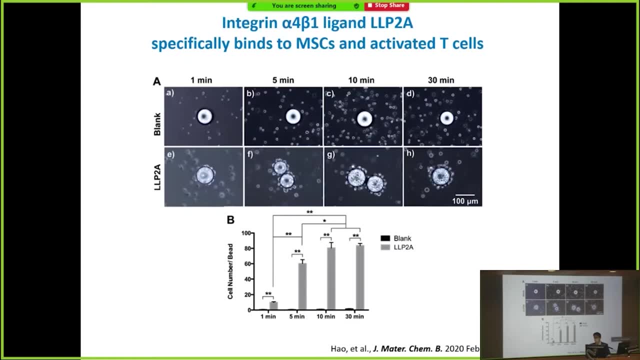 modification on the surface of a scaffold, you can significantly increase the cell binding to this medical device and also proliferation and lots of other good stuff. Another example: because we're interested in mesenchymal stem cells. we know that mesenchymal stem cells are highly expressing. 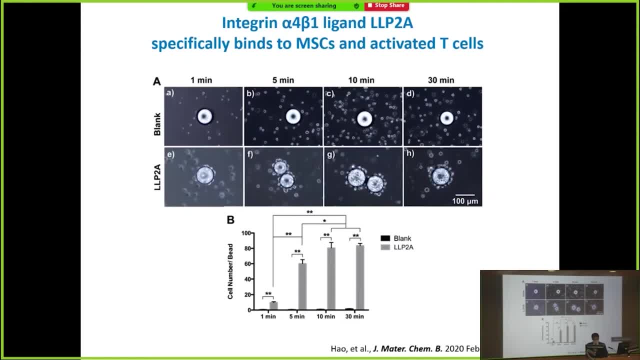 alpha-4 beta-1 integrin. We actually have been testing alpha-4 integrin ligand LLP2A against our placenta, MSCs And also activated T cells and some other scenario. actually, they highly express alpha-4 beta-1.. 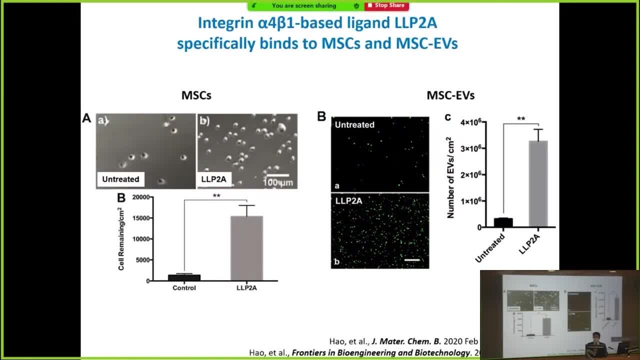 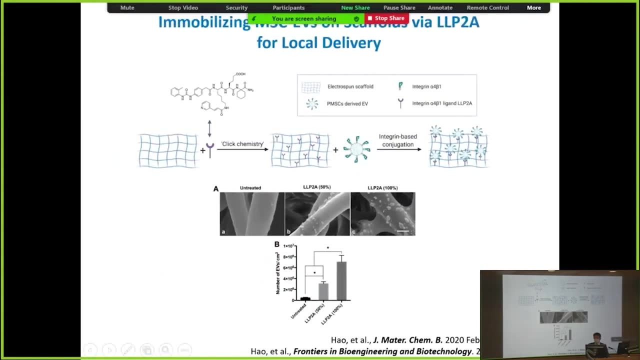 We are seeing that LLP2A and alpha-4 beta-1 integrin are able to significantly improve MSC attachment and also function downstream connected to integrin alpha-4 beta-1.. So by using this ligand, actually we can not only immobilize or improve MSC to attach. 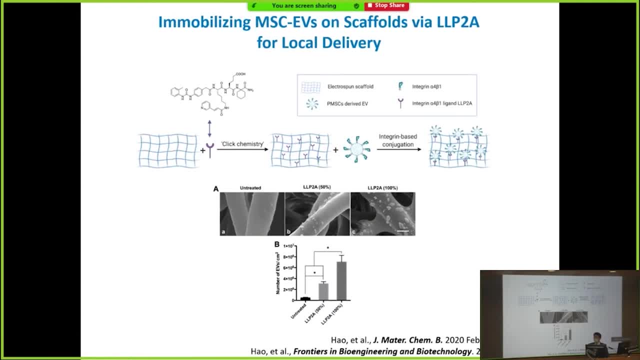 but also you can control the MSC-derived EVs to a medical device. So, as you can see in this slide, we developed a method to modify an artificial ECM surface with this ligand And then you can immobilize MSC-derived EVs. So ultimately we're making a device. 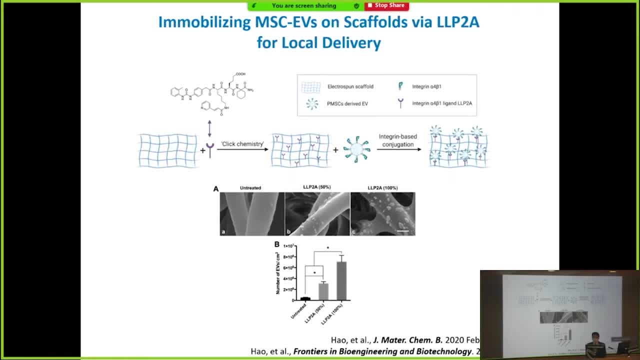 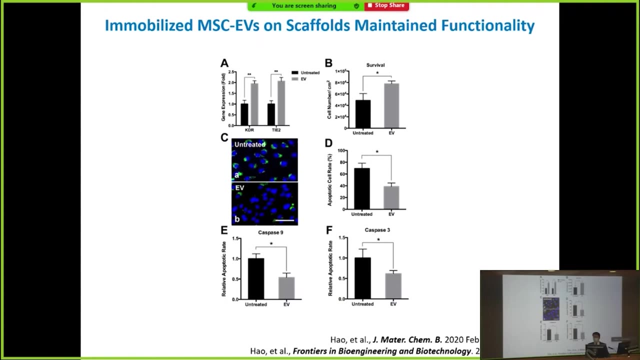 that is able to deliver MSC EVs on a local area and for sustained release. So I'm not going to go deep on how we can use this, but actually we're having several applications around this technology right now in the lab. So we are also showing that with this immobilization. 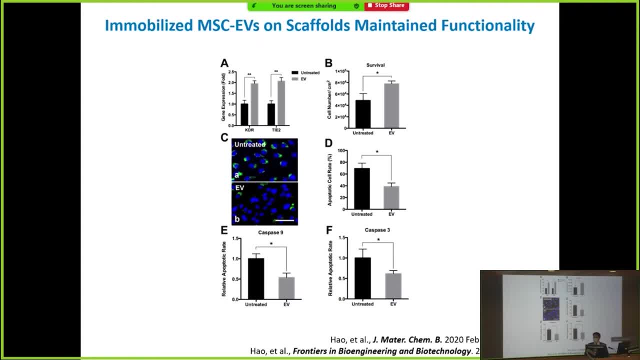 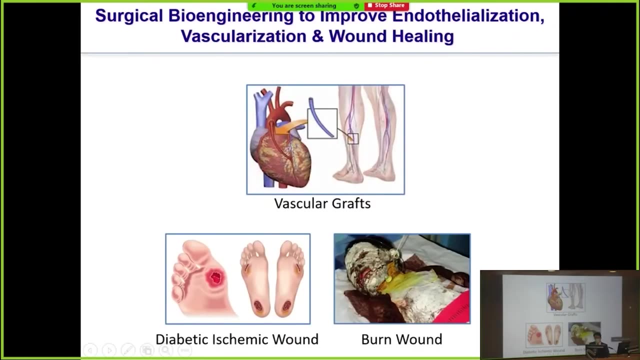 technology which can have the circulating free EVs being immobilized on the medical device surface. we are showing that the MSC EVs are able to maintain their functions after being immobilized on the surface of the medical devices. So a few other applications of the ligand technology. 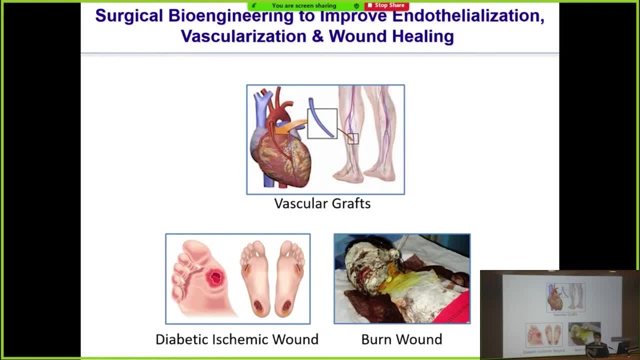 and also potentially how to motivate and also recruit endogenous stem cells and also transplant stem cells, especially endophilic progenitor stem cells, from ex vivo to in vivo. So we're using several models and disease actually very closely relevant to our surgical specialty. 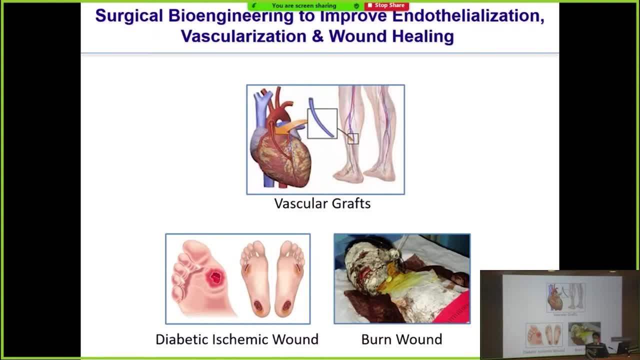 for example, vascular disease and transplant environment, for example, where hemodialysis patients are requiring a vascular graft, for example. or vascular disease, where patients require a vascular graft, and also diabetic wound, where the environment is very ischemic And so we and also burn. 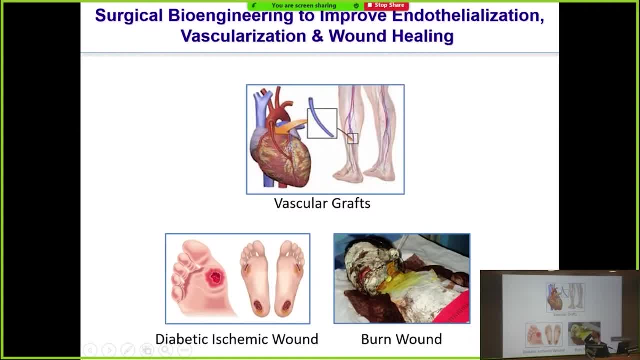 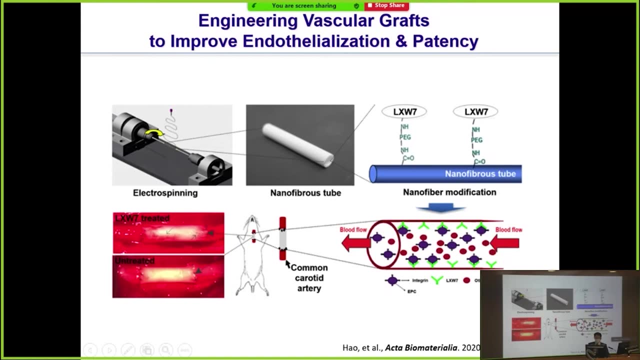 So this is. I'm giving you a few slides about each cases, how we're using our new technology to modify the scaffold or medical devices that can be applied to these surgical applications. So let's start with the vascular graft. I'm going, I'm going to go through these slides quickly. 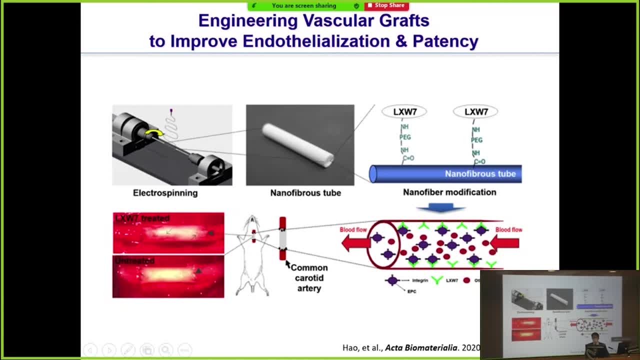 because we have published several papers about this. So the idea for the vascular graft to improve the endophilization and patency actually came from long back. long time back Because, as you know from circulation there are lots of stem cells. 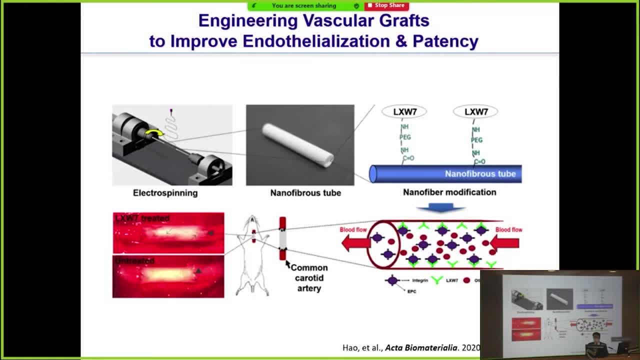 There are endothelial progenitor cells too. But how to effectively immobilize those cells or to capture those cells to your medical device surface to make them function or to become into a functional endothelium is a challenge. It's not easy because they are so rare. 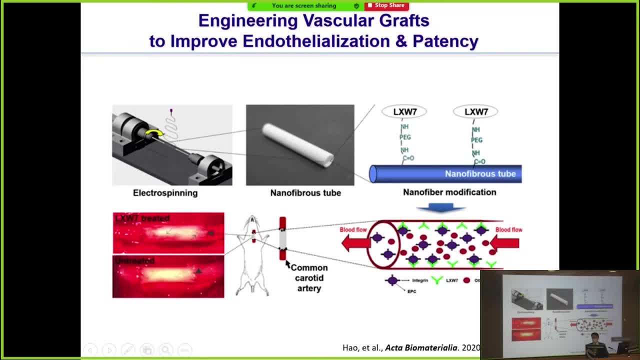 There are many other cells. So we have actually used this technology to capture this very rare population of endothelial progenitor cells, but not other cells. There are many other cells that are showing similar properties, similar integrating expression on the surface, But this peptide technology actually we developed 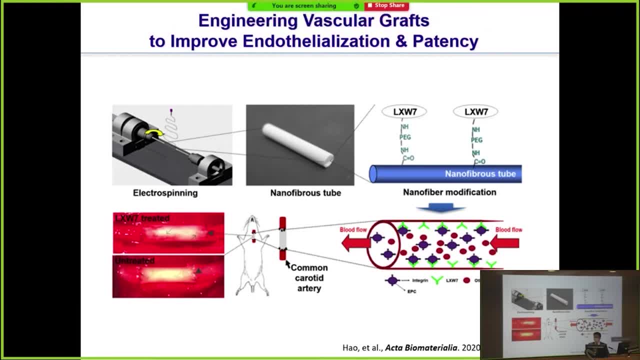 has been shown to be very specific to support endothelial progenitor cell binding and also downstream functions. So, as you can see in this slide, we are basically making our own small diameter vascular graft which is actually a target for future use in cardiac or 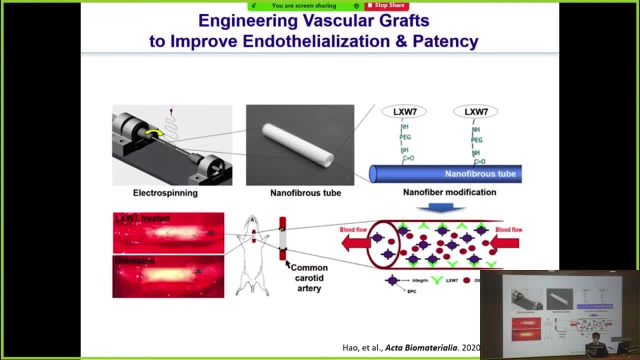 coronary artery disease, for example, But of course we can use this vascular graft for many other conditions. So we're using this small animal model- rodent rat model of cardiac artery, which diameter actually is only about one millimeter. This is super small. 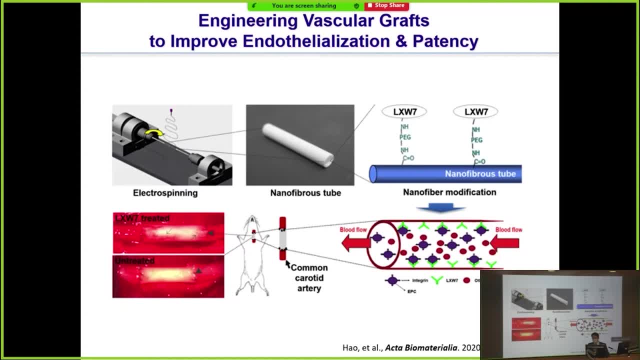 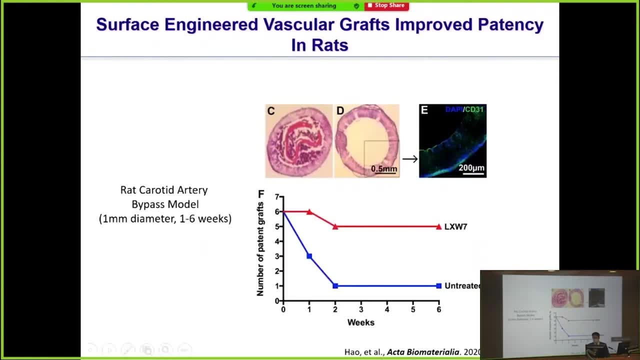 And if you don't do anything for such a small diameter vascular graft, the surface will be clogged very quickly. But I'm going to show you very quickly about how our technology can change this. This is what we did: This X-ray. 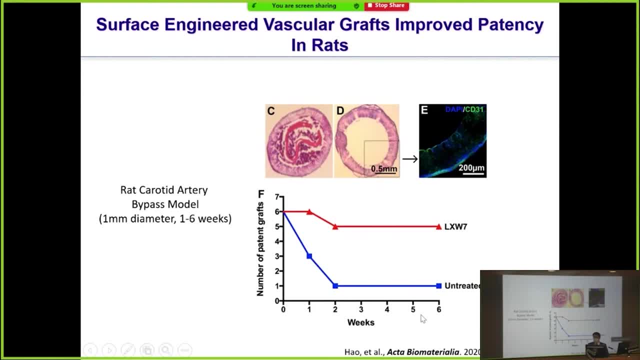 This is the first of the seven modified small diameter vascular graft. Actually, this is the X axis, is the time points per week, one week until six weeks. You're seeing a number of animals who can still maintain the patency of the graft. 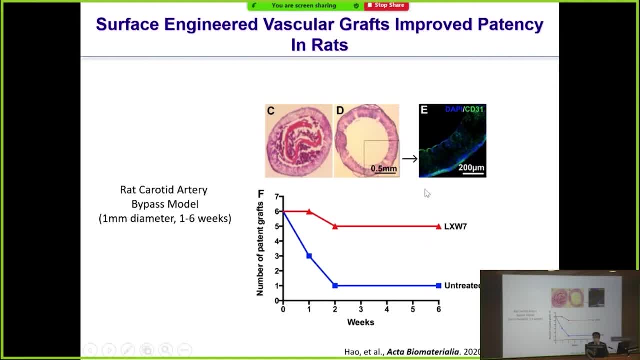 maintain the opening of the graft And, as you can see here many grafts without any modification, they're going to become clogged and blocked by the thrombosis and many other cells and tissues quickly Actually. for example, you can see the blue line here. 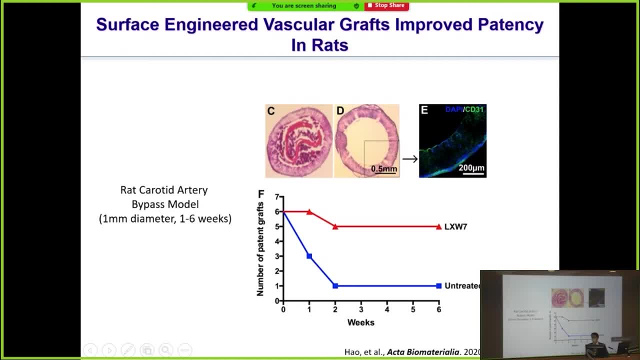 Within two weeks. actually, most of the grafts are clogged. But with this surface modification, with this technology, you can see, actually only one out of six is blocked And five out of six actually stay open for this period of time. 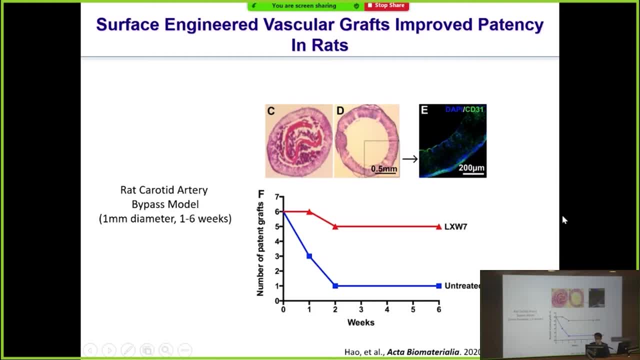 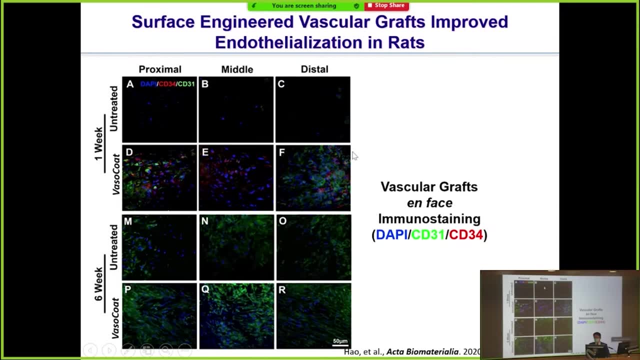 And from the histolic control analysis you can actually see that lots of endothelial cells So showing here. red is endothelial progenitor cells And green is mature endothelial cells. And this is one week The control graft And this is one week the coated graft. 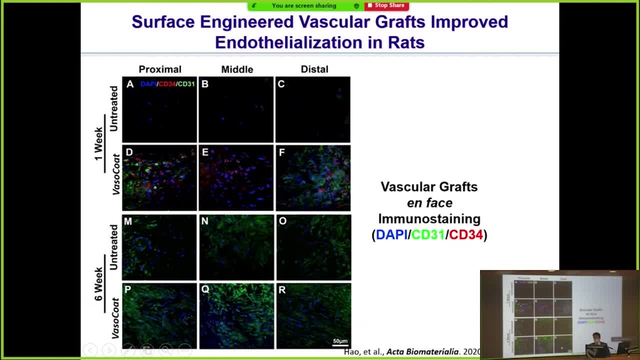 This is six weeks of control graft. This is the six weeks of coated graft, So we can see that actually the coating technology has significantly improved endothelial cell binding and endothelialization of the scaffold And now we're actually transplanting this into the large animal model. 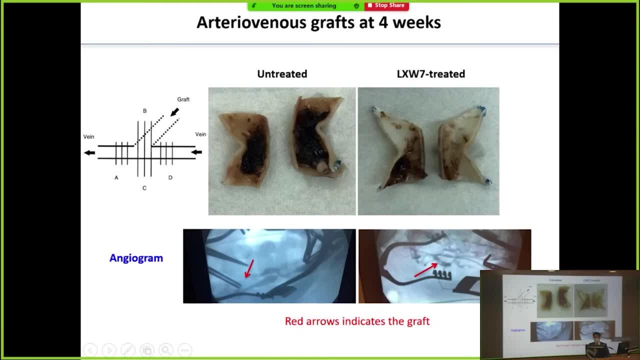 And we have done a preliminary study. We're seeing that with the XW7, we're doing this in an AV graft, so where we have the graft connected to the artery and vein in the pig model, We're seeing that with the coating, with this coating. 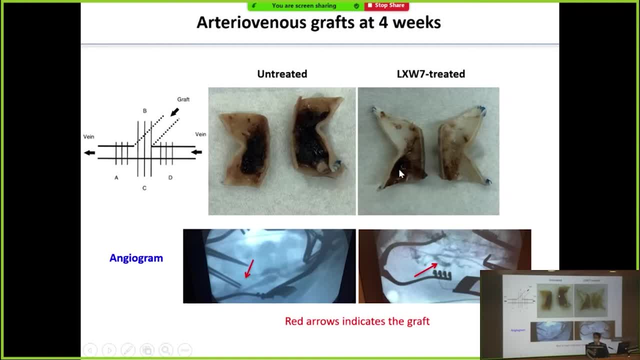 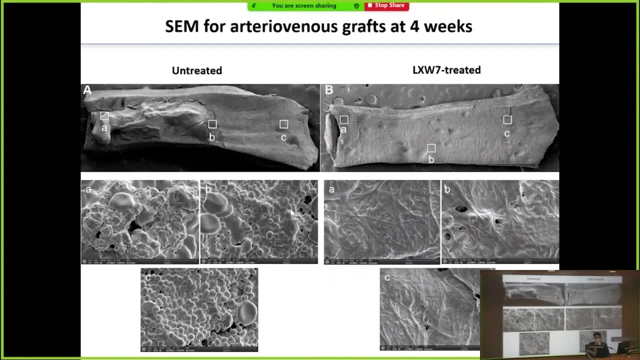 actually you're having a much better surface compared with without coating. This is the PTFE graft that you usually use in clinic And at four weeks actually, if you look at the luminal surface, you can see a lot of the cells or different stuff. 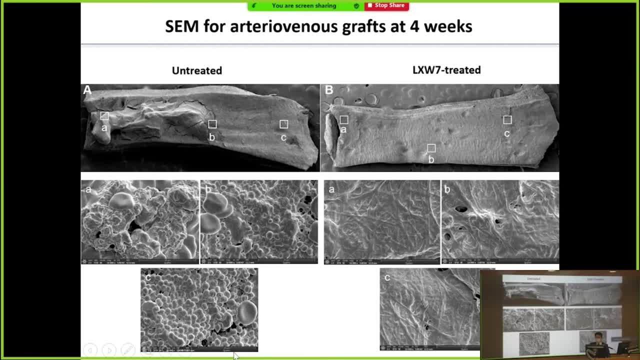 different things are attached to the surface. On the untreated surface you can see a lot of platelets and platelet aggregation And lots of red cells. It's big pie-like shaped cells. There are red cells, a lot of platelets. 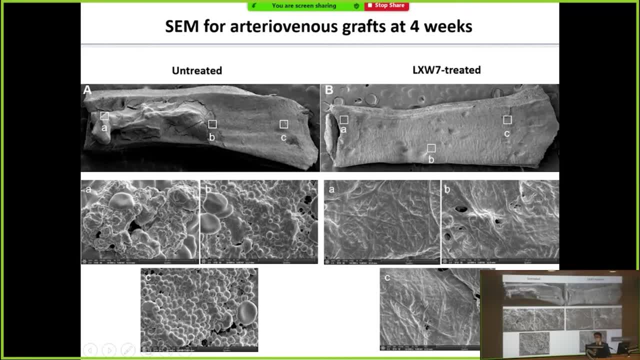 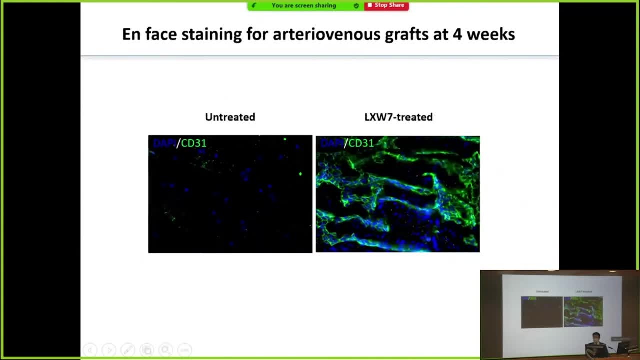 But on the surface, treated graft with XW7 technology, you can see a significant amount of endothelialization. All these cells actually are showing in bioimmunohistochemistry. They're actually having mature endothelial cell markers, the E31 expression. 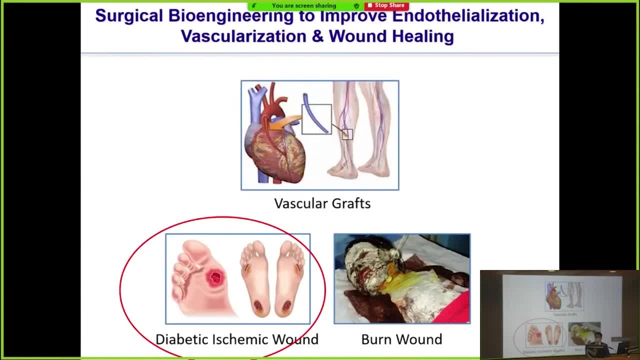 So this is very exciting. But this is a major, like a bigger blood vessel. Can we use this technology to improve small blood vessels or vascularization for new tissue formation? So one use is ischemic wound in diabetic wound- Very quick. I know all of you, most of you. 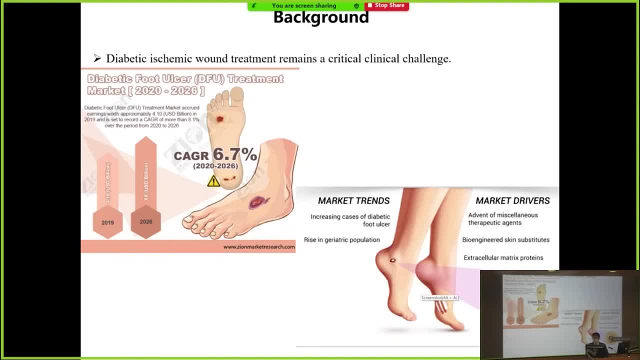 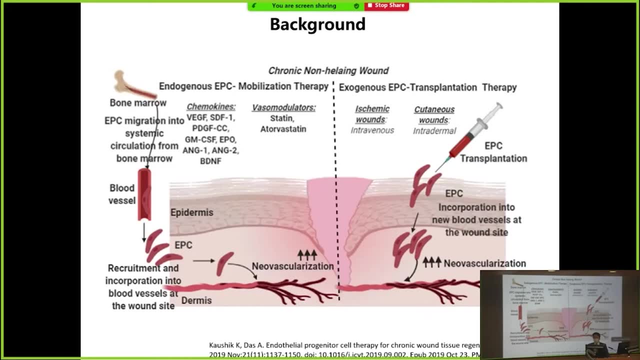 know much better about diabetic wound healing than me. There's a huge clinical need. So the key question here is: in this very super ischemic environment, how can we promote new vascularization? This is a key question, Whatever strategy you can have, if you. 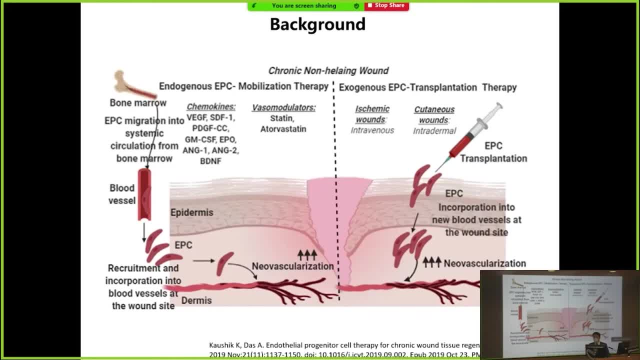 can motivate endothelial cells or endothelial progenitor cells to make a better new vascularization. that's a win. So there are different strategies that have been explored in the past, For example, endogenous EPC mobilization or different technologies to get EPC endothelial progenitor. 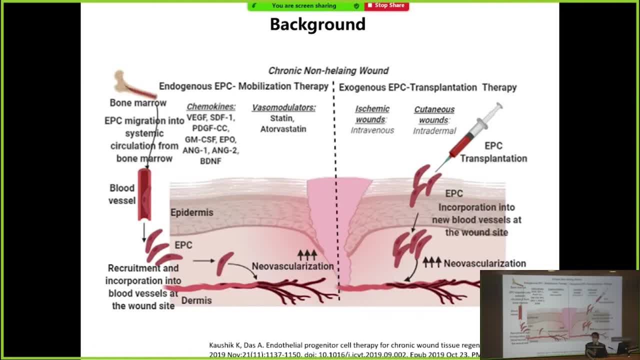 cells, to activate and to make more of them and become into functional endothelial cells and vascularization. That has been studied. And also transplantation of EPC from outside, expanding EPC to the body. So, But still EPC survival actually. 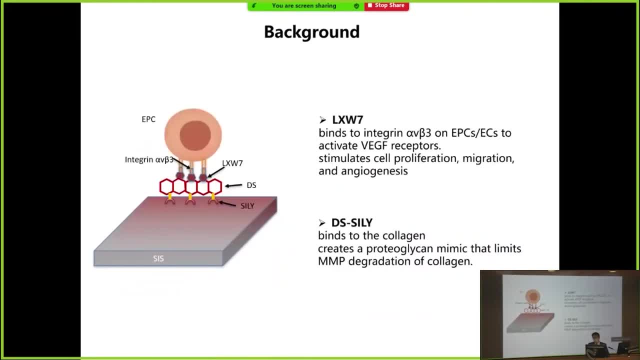 in this super ischemic environment has been a challenge. Our technology- we're hoping to develop a technology based on this technology- is to improve by providing a binding surface and stimulating endothelial cells. We're hoping that endothelial cells can survive better and also can function better. 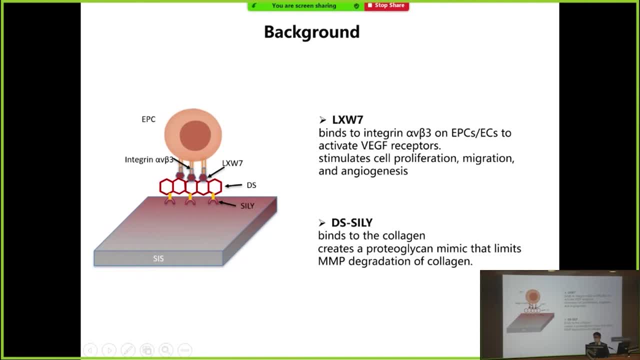 We have this SIS scaffold that you know very well about, which has been used in clinic for diabetic wound healing and many other cases, and our spina bifida research. we were replacing materials made by SIS, So we're using this clinical product. 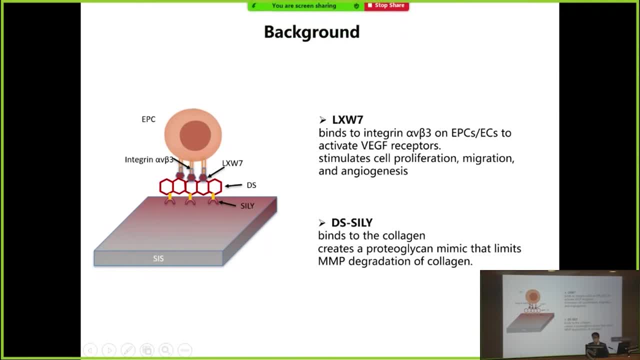 We're trying to modify the surface of SIS by using this DS-Silly XW7 technology. There's a lot of science behind this, but just to make it very simple for you to appreciate how this works, basically, DS-Silly is a large sugar chain with many side chains. 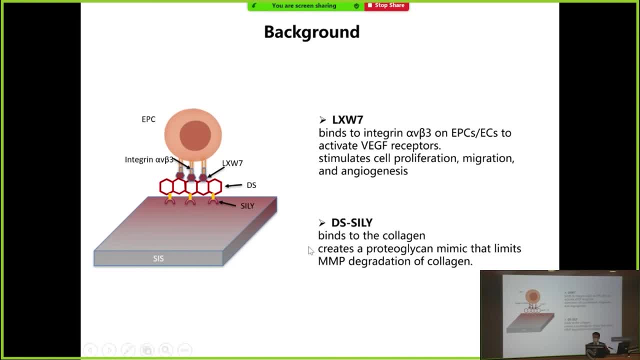 and where you can have both XW7, which is able to bind to endothelial cells, and also the Silly peptide, Which is able to bind to collagen. So essentially, we have a dual functional peptide that one hand of this molecule can bind to the scaffold. 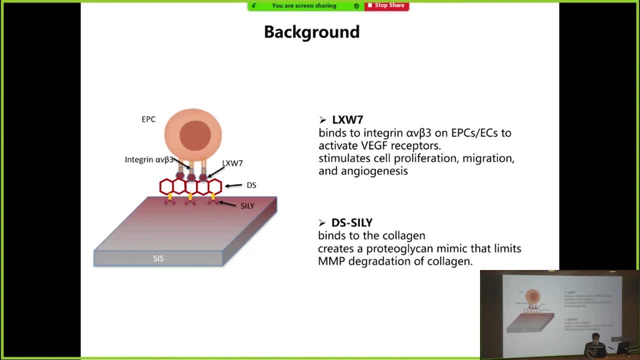 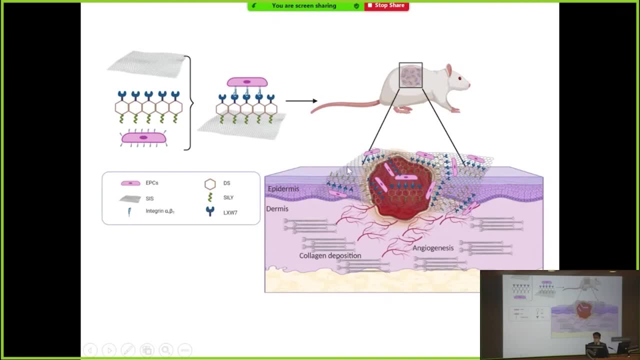 The other hand of the molecule can actually bind to endothelial cells. So by using this technology, we're developing a new product. Now this SIS is a functionalized peptide and then loaded with endothelial cells, And then we actually apply this into this diabetic wound. 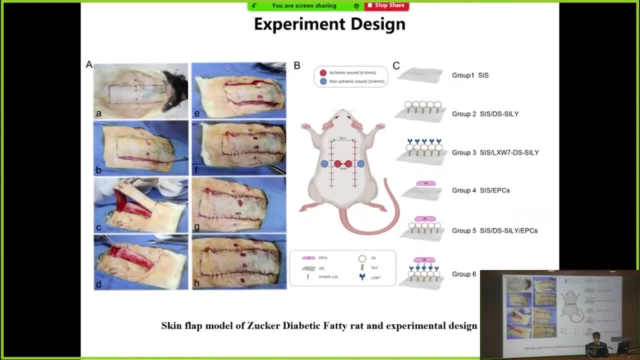 application. So in this case we start with the road and model. We're using this Zucker fatty diabetic rat, which is very fat as you can see in this picture, And they are actually having very similar physiology or pathology with human diabetic situation. 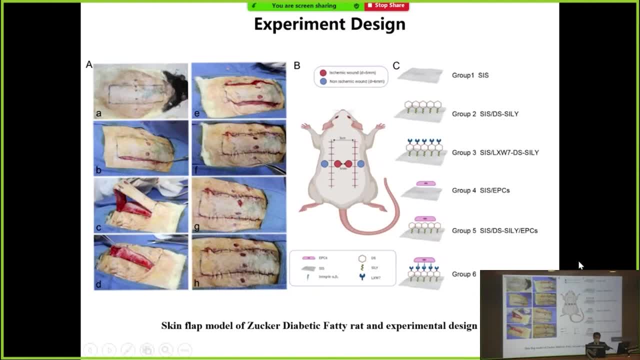 And we're making this tissue flap models with four holes, and two holes in the middle having a silicon membrane underneath, And then the hole actually is making the, the uh, uh, uh, uh uh and the the cut from this square. 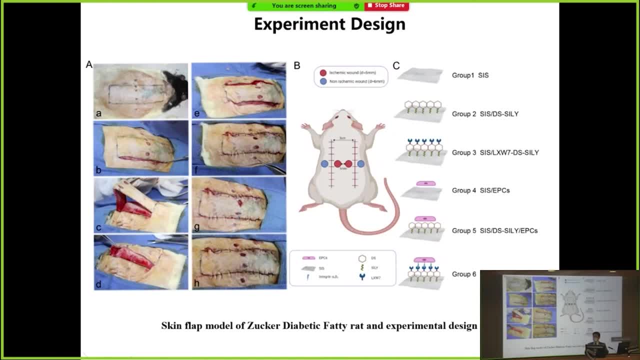 is making the blood supply from all, almost all directions of being uh limited, including from the bottom. So this middle two hole, these middle two holes, are very ischemic. We're also having these two uh blue holes on the side which have the uh blood supply. 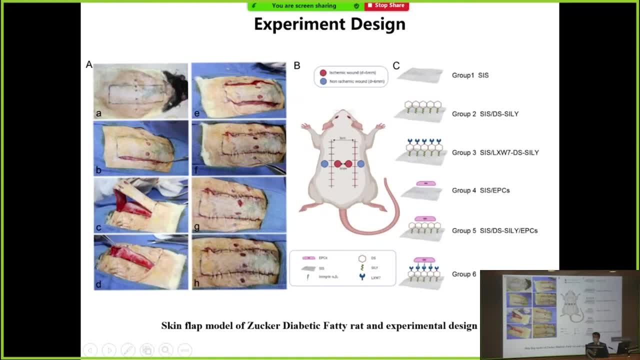 from the surrounding, only not from this cut. So this is relatively non uh uh, non-ischemic environment. So we're trying to see, see if the scaffold loaded with different molecules, these are being by itself without any modification. 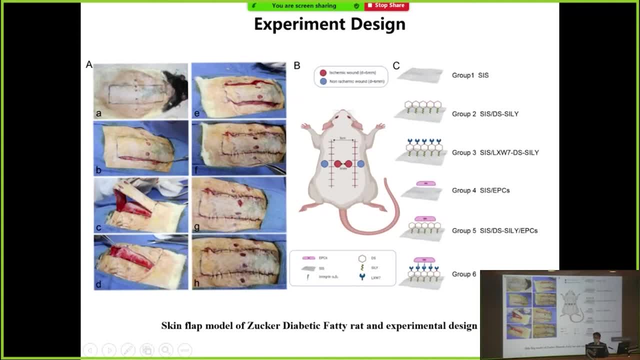 or SIS modified with DSCV and LXW7 DSCV modified SIS or SIS directly loaded with EPC or SIS modified with different peptide loaded with EPC. So, ultimately, we're trying to dissect out and see which molecule or which part of the whole device. 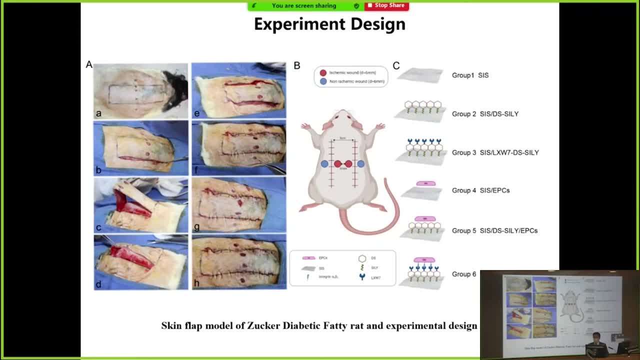 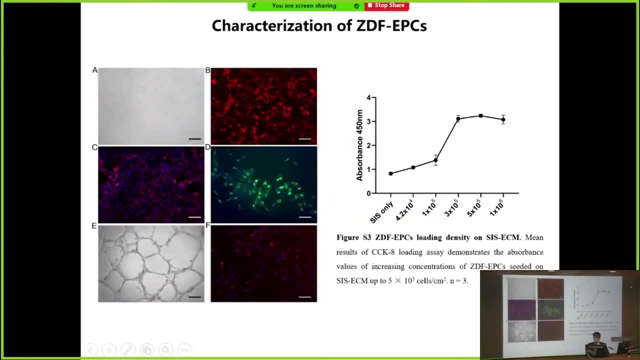 is playing the most important role in mediating some endothelial cell functions in this ischemic environment- diabetic ischemic environment. So first of all, we actually looked at ZDF EPCs. So this is the Zoccher fatty rat- diabetic fatty rat. 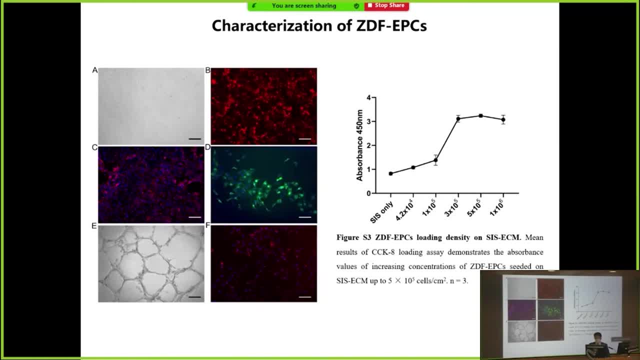 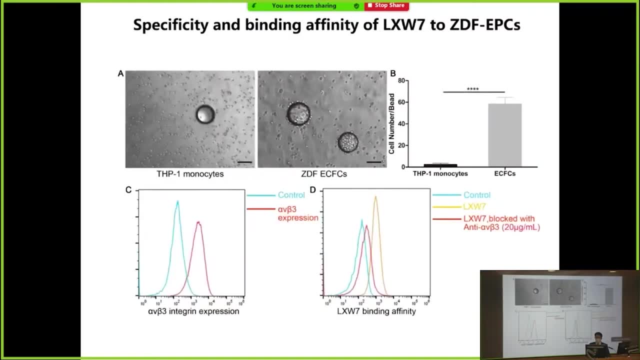 So they have isolated EPCs and they actually show we actually purchased this EPC from the company. We're showing that this EPC are similar to human EPCs in many ways, including those expression of alpha, beta and beta. 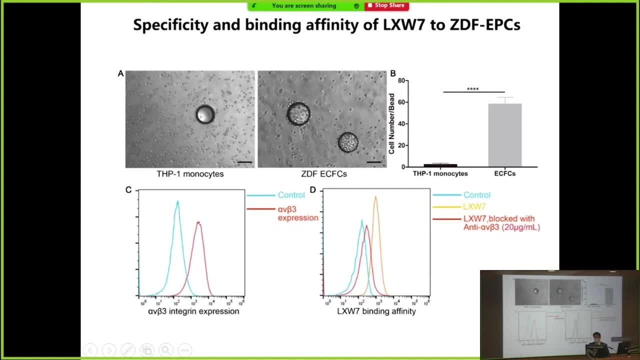 And we're also showing that alpha beta, beta, beta 3 integrin on the surface of these EPCs And we're also showing that LXW7 can actually bind to this integrin alpha beta, beta 3. 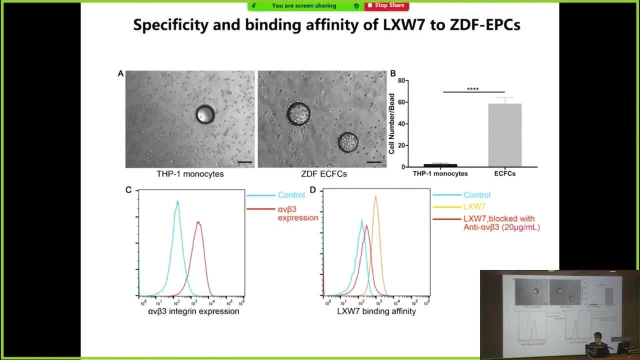 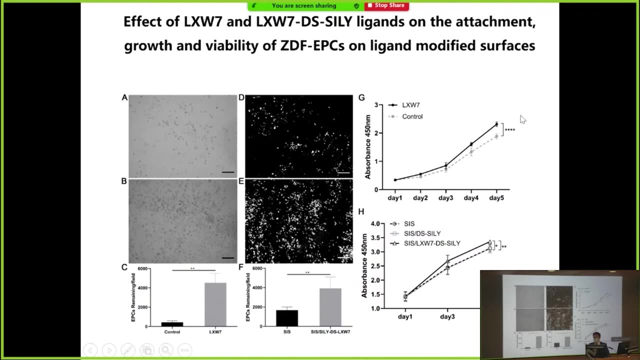 on these Zoccher fatty rat EPCs And this can be blocked by antibody of LXW7 integrin. So this shows the specificity of this ligand interaction with the cell. We're also showing that by having this ligand modification on the surface, the endothelial cells seated. 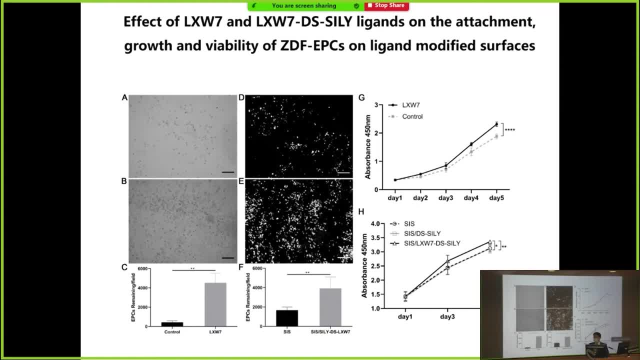 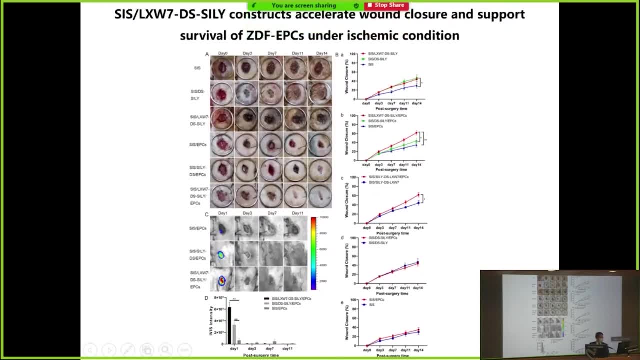 ZDF. endothelial cells seated on the scaffold can proliferate much better, Attach better and proliferate better. This is the key data. So what you can see here is that a different time point from day 0 of the middle two holes of the very ischemic diabetic wound, day 0 to day 3,, 7,, 11,. 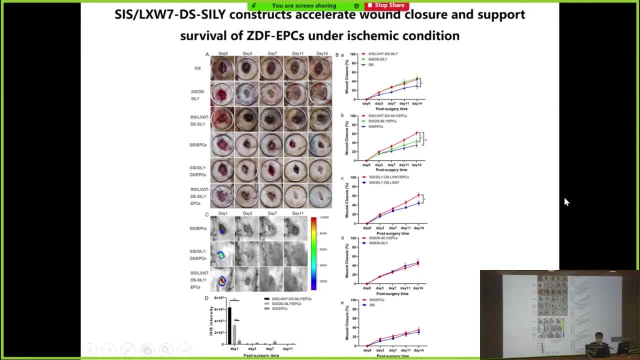 and 14.. You can see the heating rate actually is quite remarkable. You can see from this diagram showing the blue is a regular SIS And the blue is the regular SIS. The green and red are SIS functionalized with SILI. 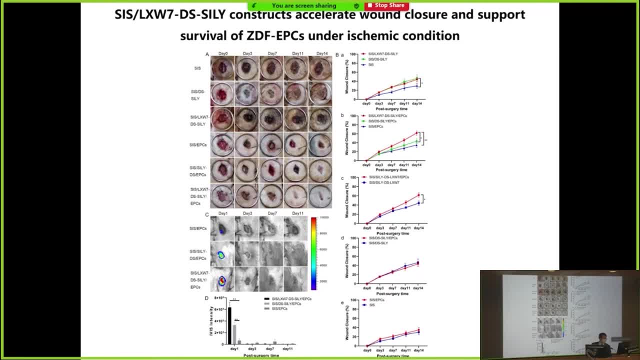 or SILI with XW7.. So you can see that actually with this, So both the SILI XW7 or the SILI modified EVs are much better than SIS only in terms of heating rate And also if you're comparing EPCs loaded. 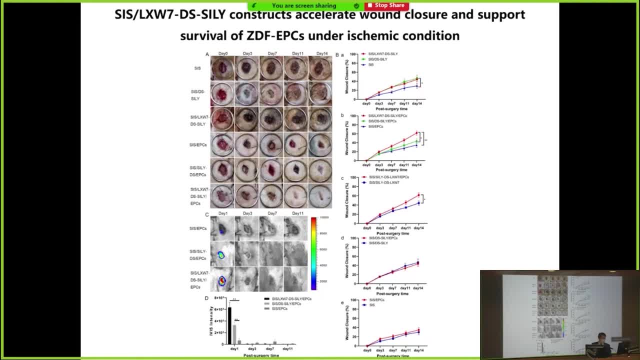 on different scaffold, with or without ligand, you can see that the red, which is SIS, is functionalized with XW7-DS-SILI, is able to improve the endothelial cell function and improve wound closure. And also, if you compare SIS functionalized with peptide, 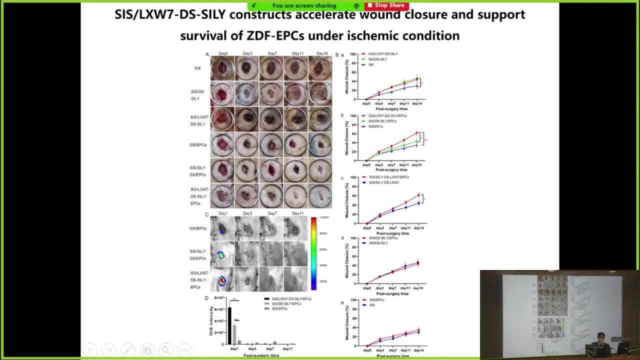 and then with EPC or without EPC. actually, you can see that with the EPC, with the peptide conjugation as a combination, you see a much better outcome in healing. All these actually are showing that XW7 is playing a huge role in modulating EPC functions. 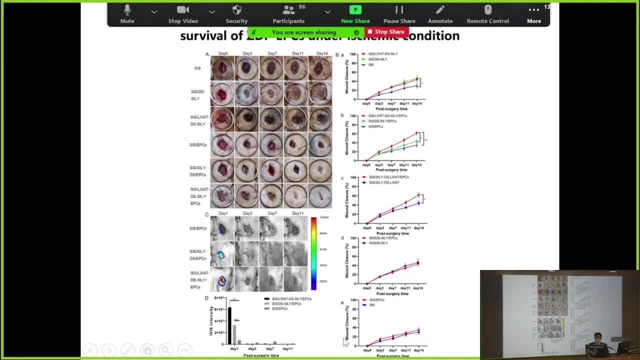 And you can see also here with the IVs to track the stem cells after transplantation. you can see at an earlier time point with XW7, actually EPCs, even in this very ischemic environment most of the cells would die very quickly. 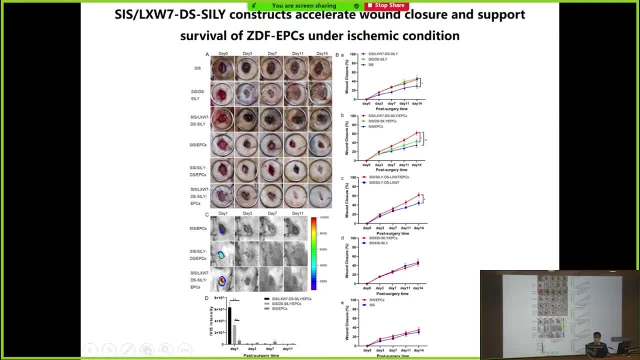 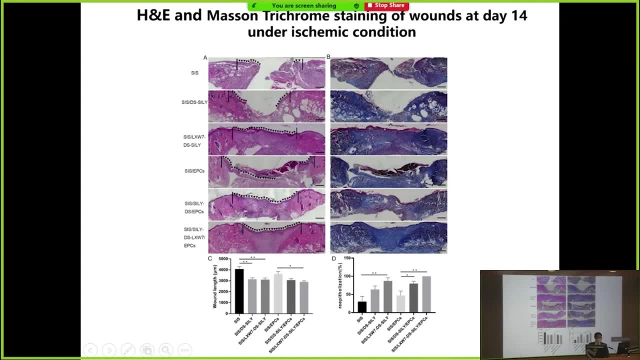 But the EPCs are able to survive much better in the environment where XW7 is provided. And then from histology of H&E and Mason's trichrome staining you can actually see from the wound length the XW7 EPC groups are or the XW7 modified EPC groups. 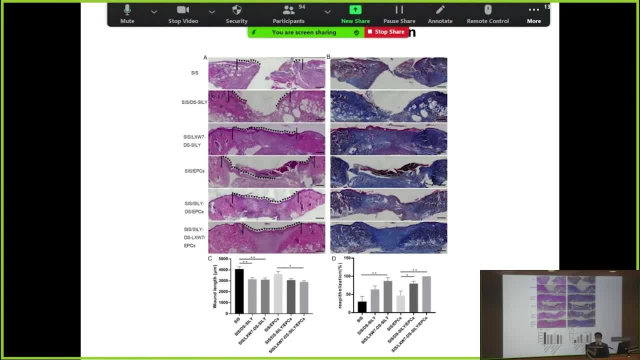 and compared with SIS without modification, loaded with EPC, the length is much shorter And also if you look at epithelialization of the regeneration of the healing. so you can see that with the EPC and XW7 as a combination, 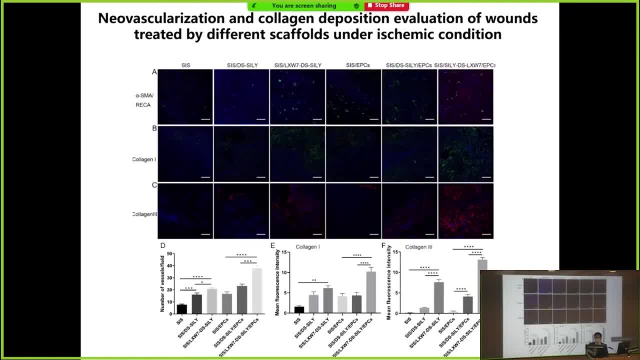 the group has the most, the best outcome in healing. So by looking at certain specific, the molecules and expression of a collagen, for example, we're looking at endogenesis. we are seeing a much, much higher density of new vessels in the group of animals treated with the XW7. 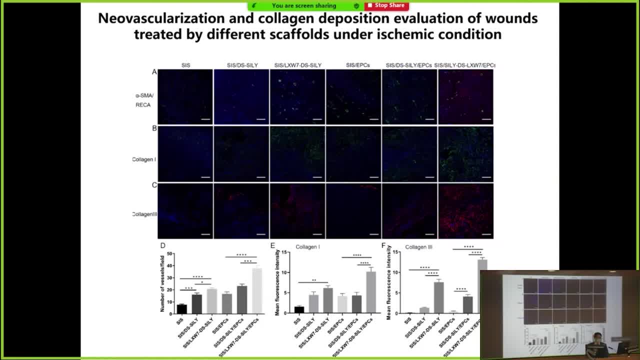 silly, DS silly and EPC functionalized SIS compared with SIS by itself. We're also seeing a much higher expression of collagen 1 and 3 in the new tissue in the groups functionalized with the peptide and the endothelial cells. 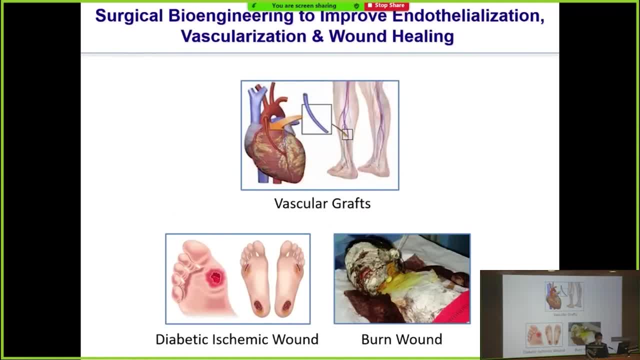 So we're doing more actually, and so burn wound actually is something that we're actually studying right now. I don't want to overwhelm you too much. We're actually establishing the model. We're trying to see how we can use this technology. 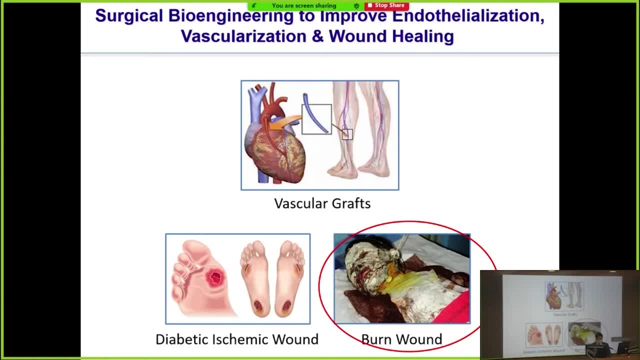 to increase new vascularization for deep burn wound healing as well. And of course, there are many other potential applications too, for example, how to increase the vascularization with any medical devices. So we're looking at a lot of different devices for different tissues like bone nerve, other tissues. 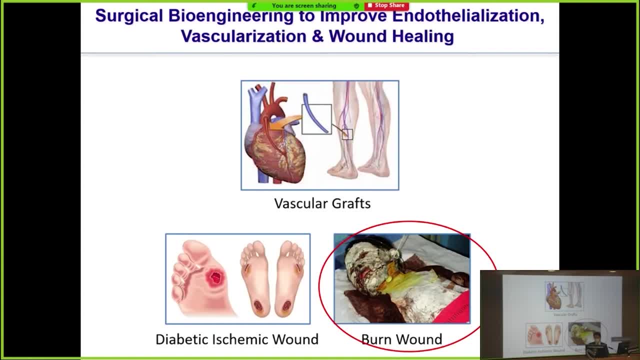 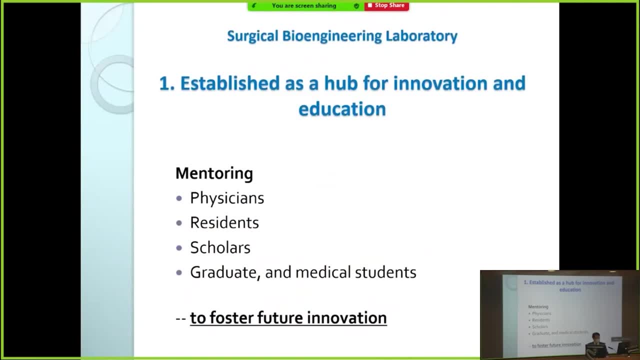 Actually, there is a huge potential for us to explore how to apply this technology, So I'm going to spend my last several minutes to talk a little bit about the lab and the resources that we can provide to the department, especially to the young trainees. 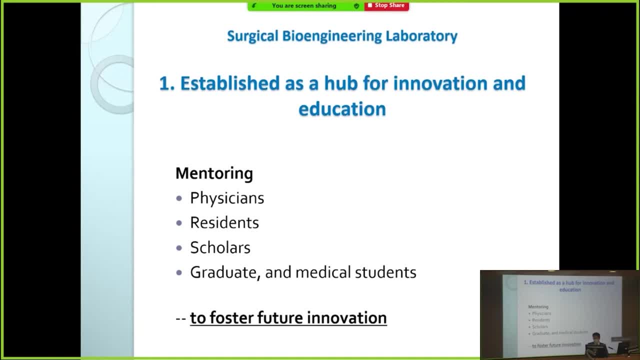 And so we are actually this lab now, with the great effort from everybody who has worked in the lab in the past decade. now we actually have really established this lab as a hub for innovation and education. Now we are providing training opportunities to many, many trainees from different levels. 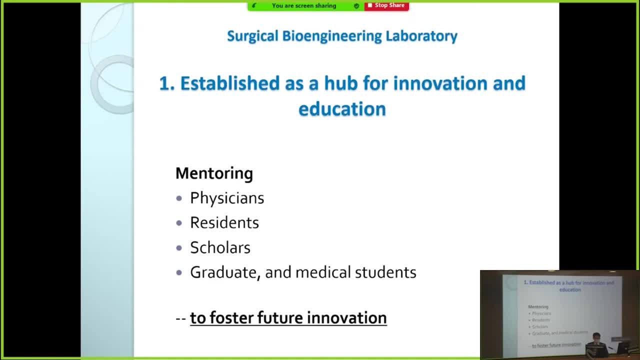 including some faculty and residents and scholars and students from graduate school and med school. So we are very proud of this And we are welcoming more trainees if you're interested in joining the lab. if Dr Farmer can get us more lab space, 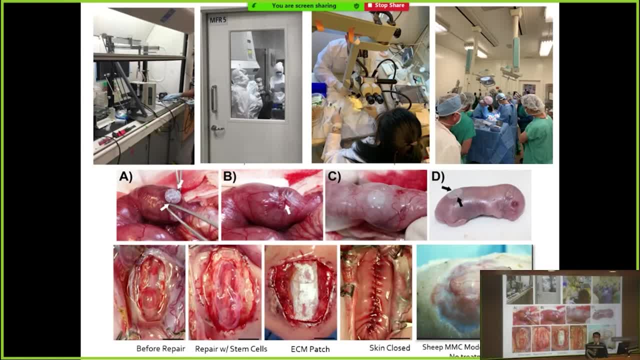 And We do have lots of expertise that can help the trainees to understand how to translate the technology into clinical application. We're having the Biomaterial Manufacturing Center, GMP or Cell Culture Team, and also small animal models, large animal models, surgical models for different diseases. 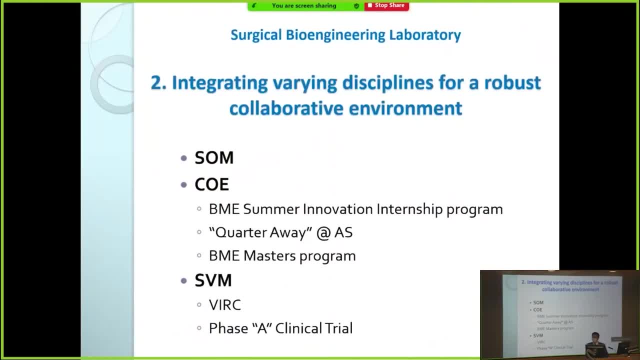 We're also really establishing a very collaborative environment. As an example, we've been really closely working with different departments across the School of Medicine School and also other departments from College of Engineering and also the vet school. We're really proud The team science actually works so well. 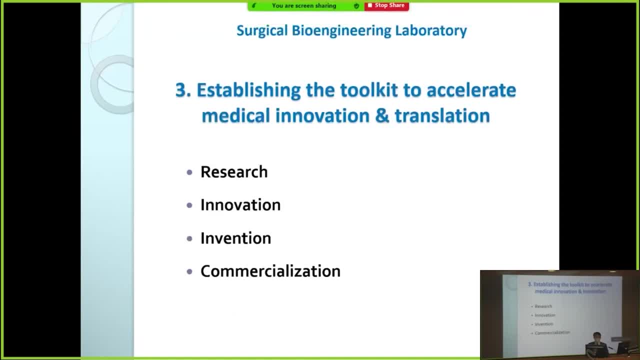 in many of our projects, And we're expanding the potential application to many other diseases and indications too. So, lastly but not least so, we're trying to see how we can develop new technologies that can be translated from the lab, from the bench, to the bedside. 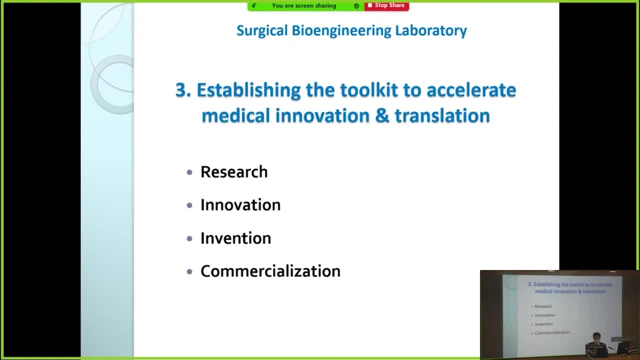 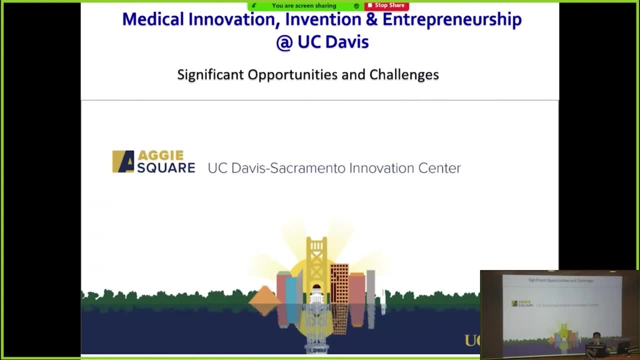 and also the translation. So we're trying to see how we can develop new technologies that can be translated from the lab to the bedside, and also the translation of this new technology into commercialization, potentially So with the Aggie Square. actually, everybody is excited about the potential. 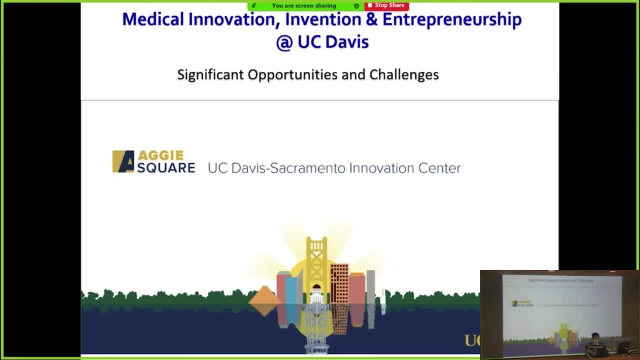 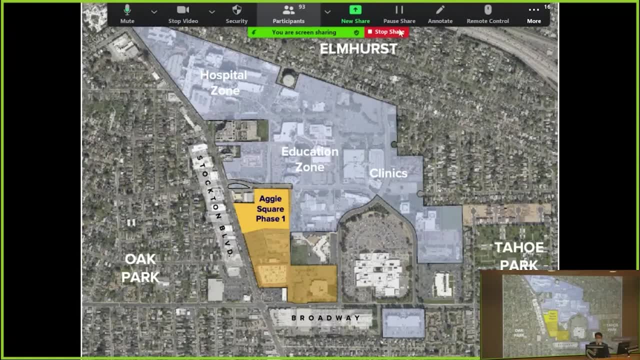 I think having more people to be excited and enthusiastic about surgical innovation and invention and commercialization- this is going to be a huge deal for our community and not just for UC Davis. As you can see, this is the older picture of the first phase. 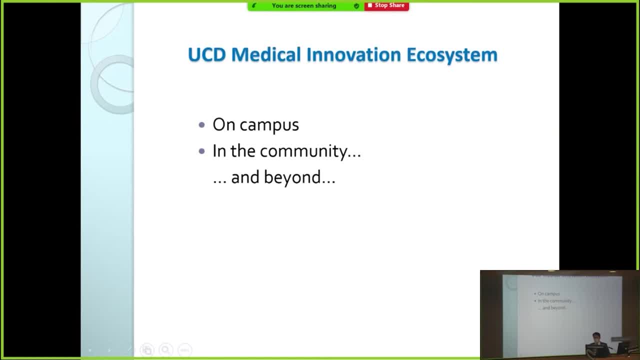 of Aggie Square. I think you know, with all the innovation work that all at large our group is doing now is going to be a. we're going to have a big impact in our ecosystem. So last slide, I'm going to give a shout out. 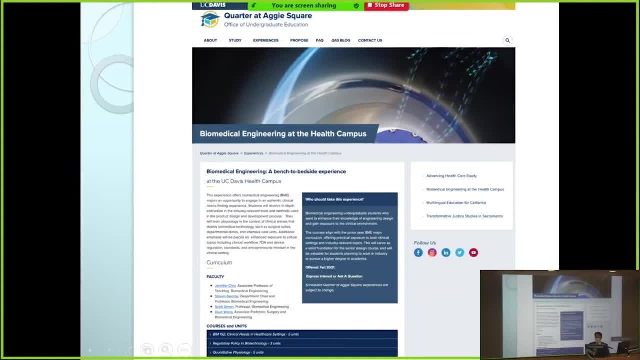 to our quarter Aggie Square program that has been supported by the provost office. So one of the programs that actually one of the first programs that got approval from the provost office, is the biomedical engineering team And I'm going to give a shout out to the biomedical engineering team. 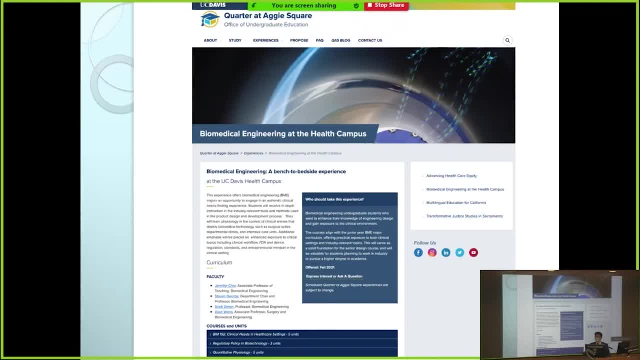 at the science on the science campus by looking at the collaboration between our department and biomedical engineering and several other medical departments- surgical department, ICU- to basically to provide training opportunities for undergraduate, BME undergraduate specifically here And also to hopefully we can get some research workforce over here. 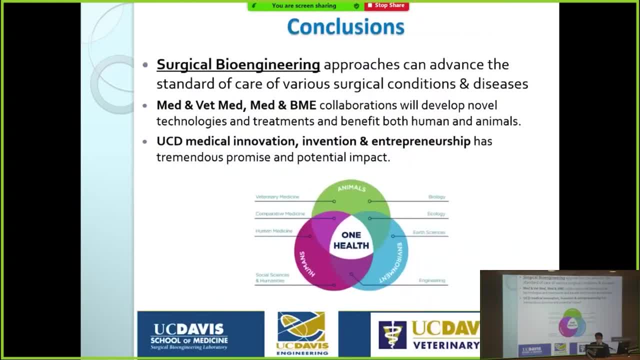 to know more about our medical research and to help our research program too. I'd like to say, as you, I'm hoping you are convinced that surgical bioengineering is making a big progress actually in improving the patient care for different diseases and also the collaboration between the med school vet school. 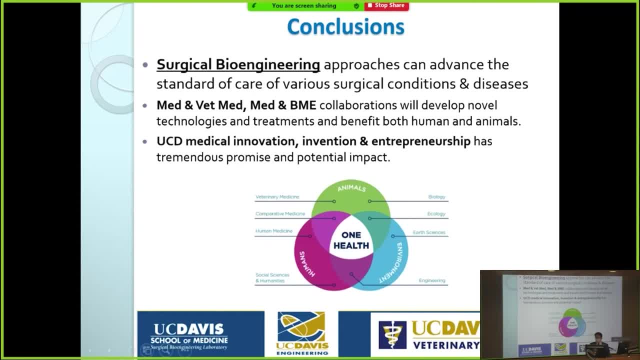 and college engineering school, So we were able to make, develop new technologies and make many innovative treatments for human and animal patients, And also entrepreneurship, invention and innovation is very important. This is really exciting and it's growing fast And with that, thank you very much for your attention. 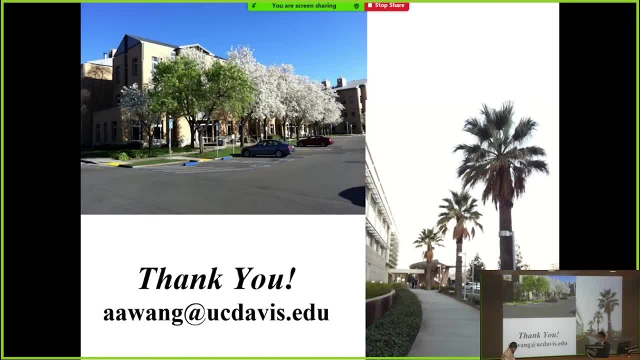 Well, Ai-jen. thank you very much And I apologize for being late. I think you can see I brought the stem cell delivery device. We were just training the OR. Dr Hirose is going to be starting a clinical trial with one of the devices that you and we have developed together. 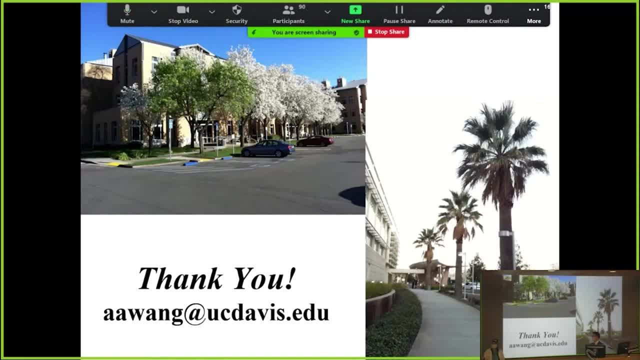 Some people have. it hasn't gone unnoticed that that's really a wine carrier. It's kind of a California version of stem cell delivery device, And you can tell we're not a very sophisticated company at this stage of the game, that's for sure. 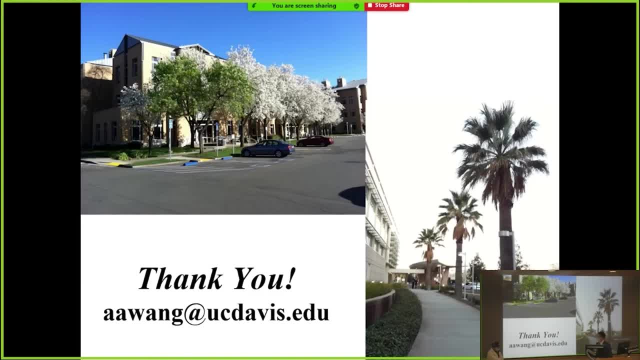 But, Ai-jen, I'm really proud of all the work you've done and really the collaborations that you've built with so many people across the department: Our plastics colleagues, our transplant colleagues, our trauma colleagues, our burden colleagues. There really are so many- an unlimited potential. 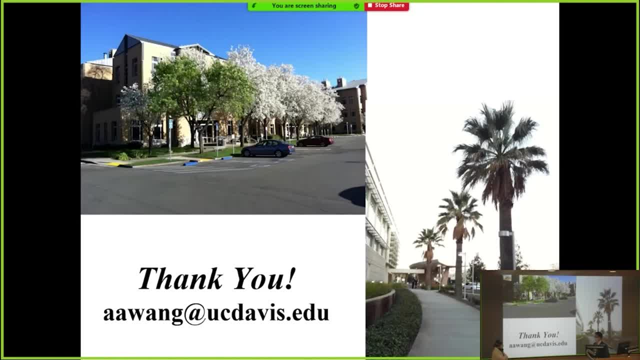 for the areas where tissue engineering and the kind of biomedical engineering that you do can have impact. In fact, now you're collaborating with some of our cancer colleagues as well, So I just want to open it up for questions, And Manny says he's got a bunch from the audience there. 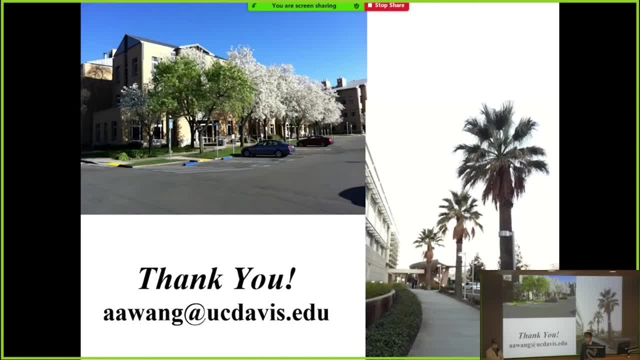 We'll start with the audience for the first time, the video audience. Yes, we have some comments and questions. We'll start with Dr Ian Brown. His comment is fascinating. Specifically, in trauma, ischemia and reperfusion, injury is a big and possibly underappreciated culprit. 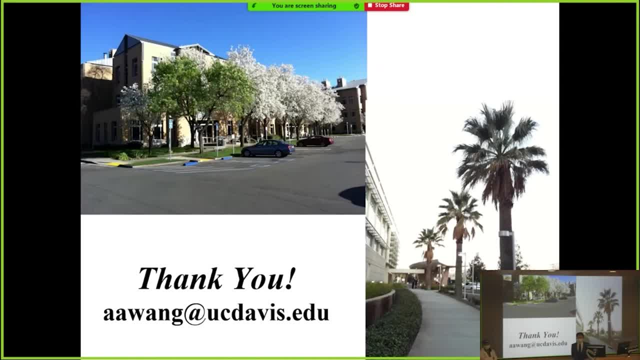 in poor outcomes. EVs have been seen as a culprit in many cases. as EVs released by ischemic gut tissue, It can potentiate pulmonary injury, for example. However, within the last few months, one group has been able to condition vascular endothelial cells. 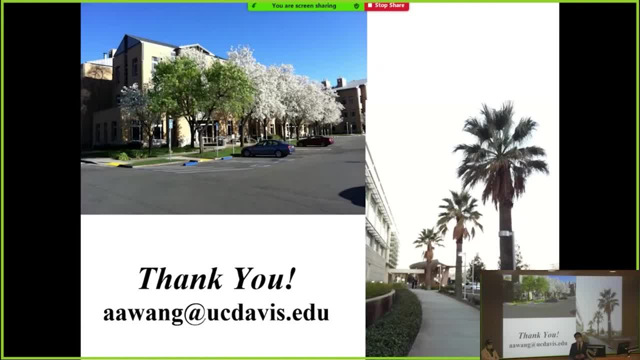 to generate EVs that can protect cardiomyocytes from ischemia and reperfusion injury- Likely a ton of potential application for vascular transplant, plastics and trauma surgery. We'd love to see this applied in animal model of riboa and vascular anastomosis. 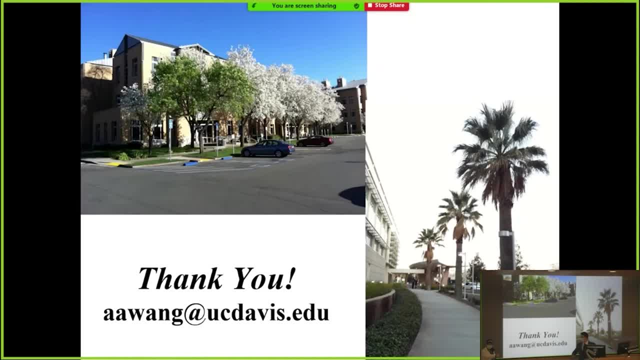 Good job, man. And then Missy Humphreys. Dr Humphreys asks when will this technology be available for us to try it in patients with diabetic foot wounds? Yeah well, Dr Ian Brown made a great comment. 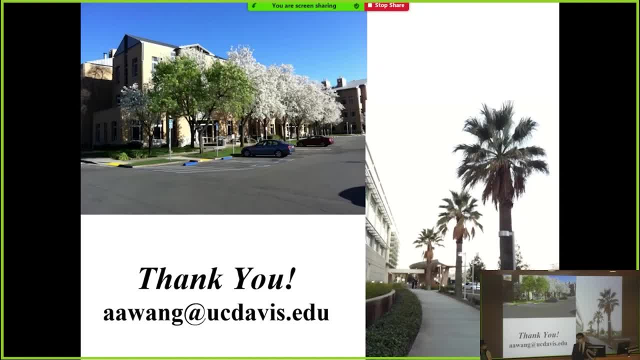 And actually I'm aware of quite a few new technologies around this EV for improving new vascularization In our own lab. actually, I don't have the time to talk about that. Actually, we do have a little bit of information that we can share with you. 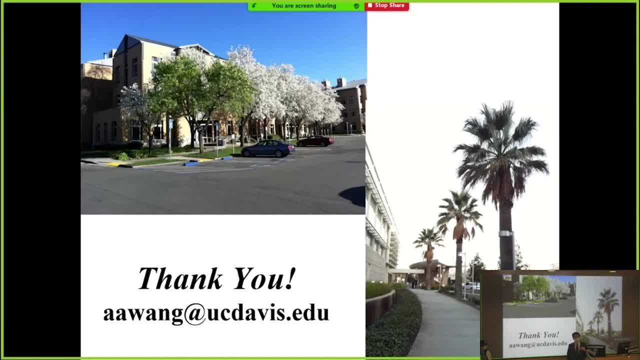 Actually we do have a subgroup who are developing EVs and engineered EVs for vascularization-specific applications, So potentially we are currently actually working with the high-limit ischemia model. We're interested in cardiac ischemia as well, because the general concept really is that EVs 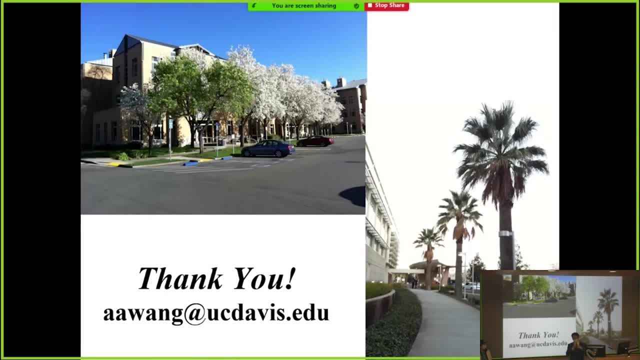 by having all those microRNAs internally in the nanoparticles and also lots of proteins on the outside of the nanoparticles, they can really be engineered to mediate new vascularization. we're seeing pretty promising results. So for Dr Humphrey's comment actually. 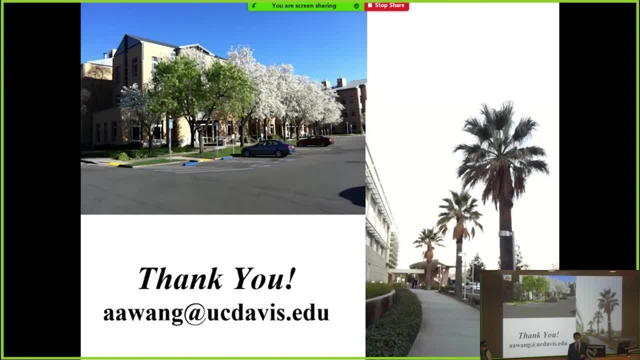 we are actively developing this and we're seeing very positive results. now I think we probably want to see how this technology will be for a couple of things before we can really translate into the clinical situation. One is that, from a product development perspective, 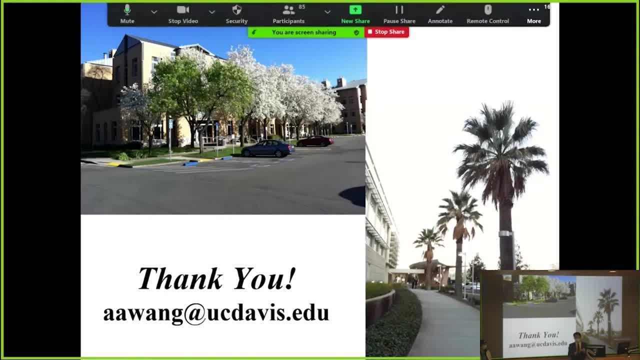 how to really control the quality overall and synthesize all the components- Actually it's going to be Eventually for surgeons. it's very easy to use, but from the product development there are quite a few steps that we have to work out. 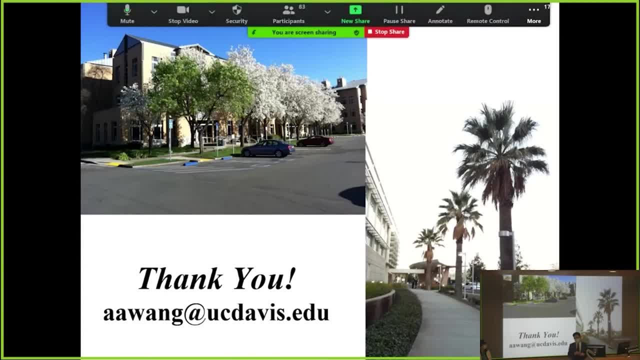 But overall actually the preliminary study is very promising. We're hoping with our expertise now in interactions with the FDA and stuff like that and also collaborators from other medical device development enterprises, so we could potentially move this quickly. Hopefully the next step would be. 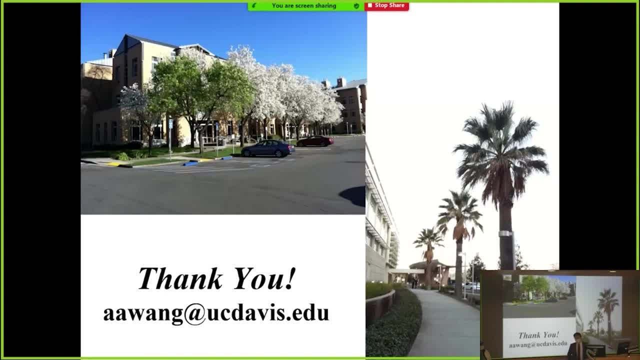 generating enough data to talk to the FDA from the regulatory perspective and getting approval, and we may be able to do some clinical trials in the near future. Quickly probably means five years, But it's amazing how long product development really does take in working with the FDA. 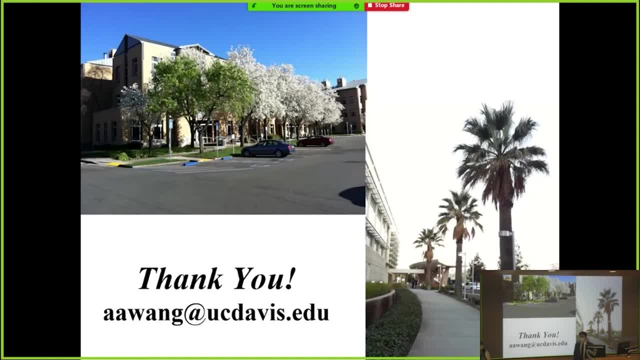 One more. Dr Greenhalgh asks: is an EV really a man-made virus? Do adrenal, Do viral delivery systems work as well? Adenoviral, That's interesting. I don't know very much about that, but I'd like to know more. 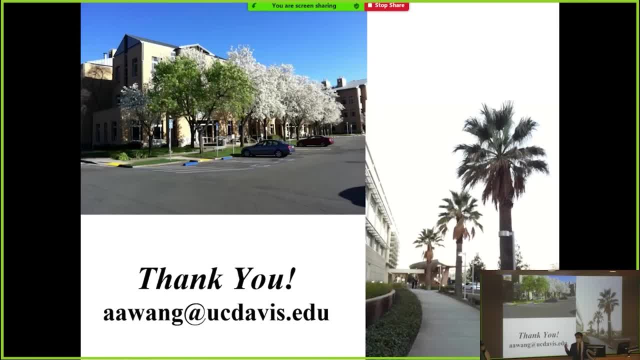 I think EVs are really. They're nanoparticles. You can consider them being a drug delivery, like a D-POT, so which can be applied into different things and you can load different things inside. It's very versatile, I would imagine. yes. 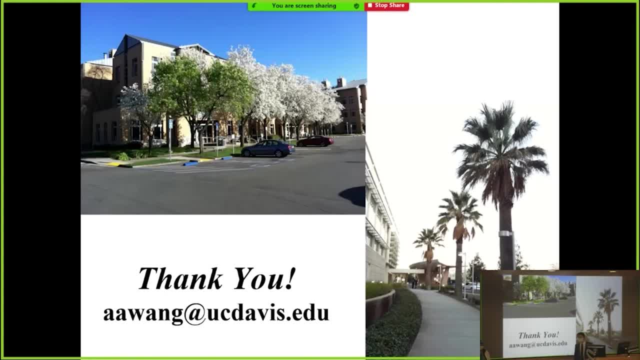 you can apply that to different applications. actually, I'd like to Just fascinating work. The issue of trying to deliver specific components to different specific areas based on attachments has long been, you know, the holy grail of trying to cure vascular problems. 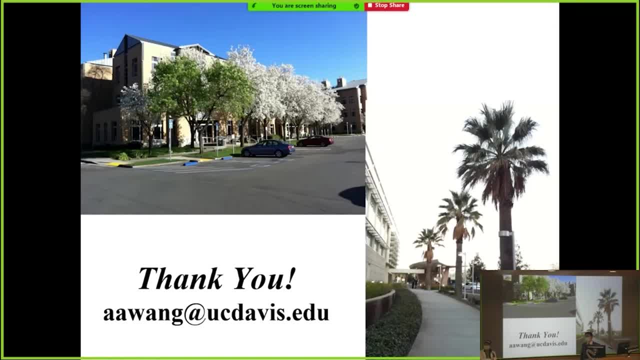 without a question. I just have a question of these EVs. Is there a catalog of the naturally occurring EVs that exist in the body? I mean, does someone catalog that? How many are there? Oh my God, there are a lot. 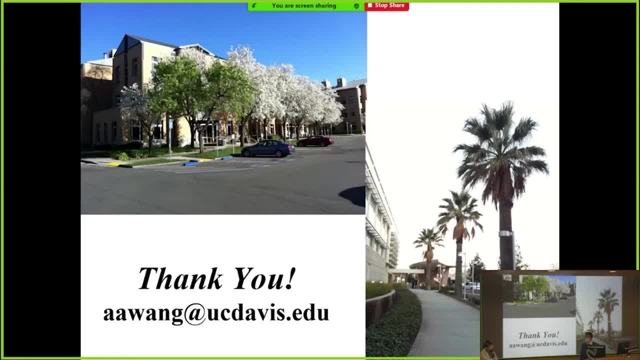 They're so small and there are many, many and every cell, all the cells, they can make EVs. So, as you can imagine, there are many cells in the bloodstream. There's many more EVs in the bloodstream too. 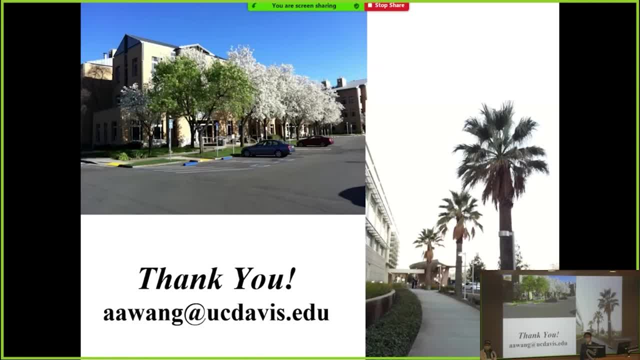 So many? I don't know if there's a number. So is the primary effort to build your own EV or to find a naturally occurring EV? Right, That's a great question. So I think from natural occurring EV. much research is ongoing about biomarker discovery. 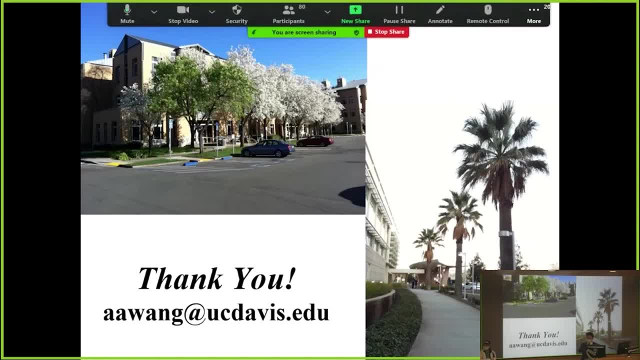 because different cells are making EVs and they are secreted. They're usually from biofluid, like circulation in purple blood, for example. You can identify those naturally occurring EVs, like cancer-associated or some type of cell-associated EVs, by certain markers. 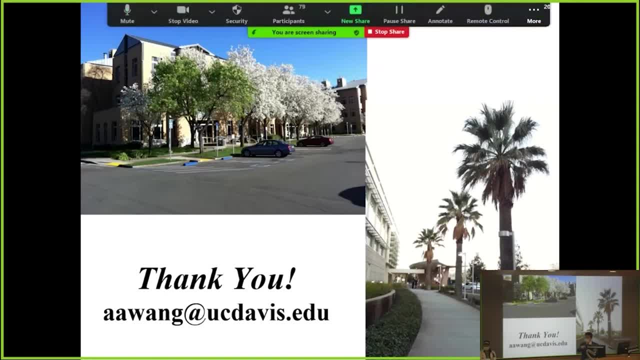 You can actually potentially identify the source of the cells and so you know more about the disease. So that's naturally occurring EVs In our case. actually, we're interested in naturally occurring EVs as well, because they're so important for different indications. 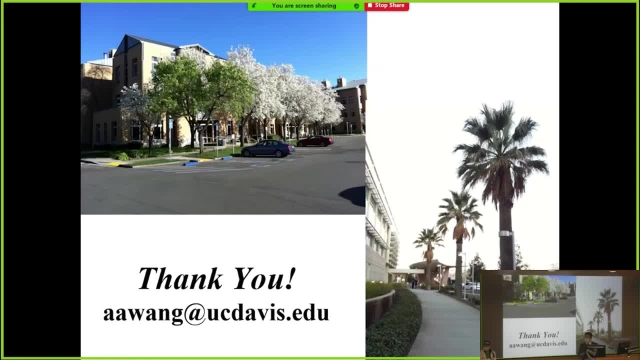 like cells in ischemia. you know cells at apoptosis. they're going to make different EVs, So we have ways to identify those EVs. You know. you can actually understand what EVs are indicating what kind of situation. We're also more interested actually. 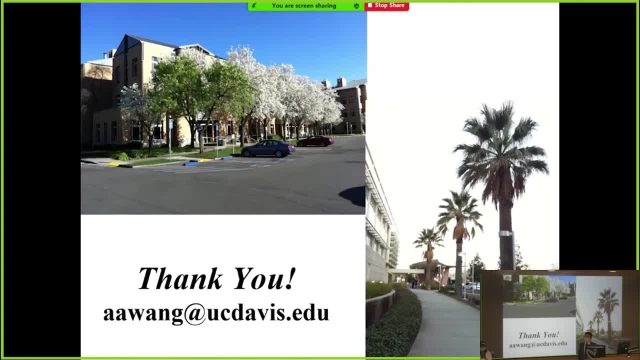 at this moment, with the limited manpower, we're more interested in developing EVs as therapeutic, So you can control the culture condition, control the cell status, control the product, so they are empowered with therapeutic potential for specific applications, But potentially both really. 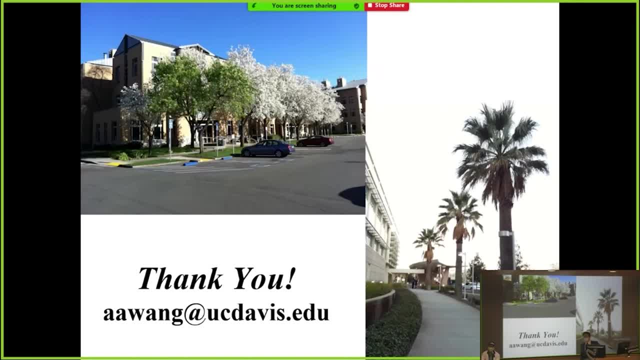 All right, we'll go back to the video world and then Dr Raskin. So there's a couple questions online, but first with Dr Brown. have you looked at scaffolding in irradiated tissues? Scaffolding in Irradiated. 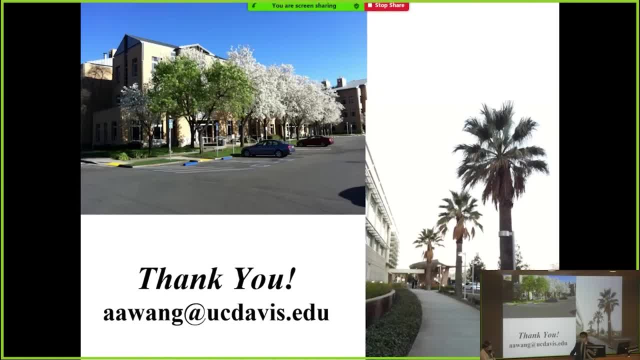 Irradiated tissues? Oh, irradiated tissues for wound healing? Wow, yes, that's one of the topics that we have been discussing. collaboration with our radiologists- actually collaborators, yes, So by promoting new vascularization, the proposal actually we put in. 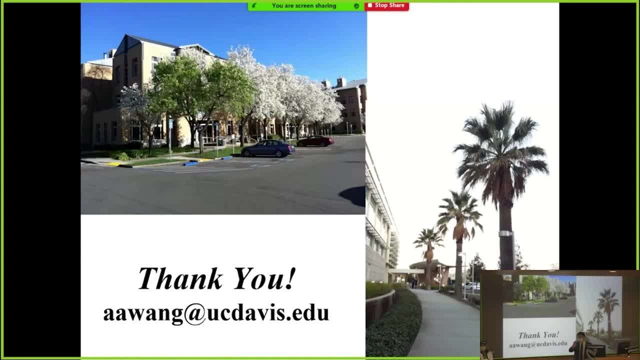 we didn't, but we're very interested in writing R1 on that as well, to promote endothelial cells in a very bad environment to make new vascularization. Yes, the short answer is yes, We're interested. We haven't done it yet. 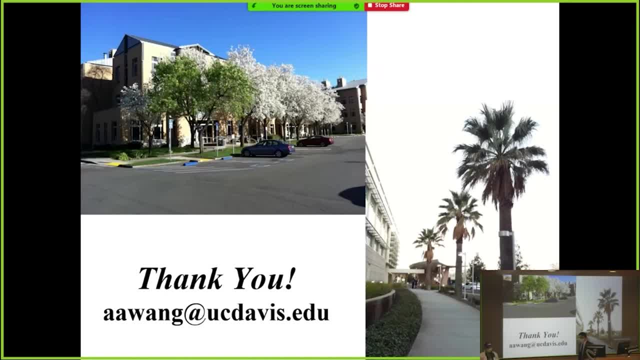 More money, more space, more lab residents. Yeah So, Dr Wang, what a fabulous talk. I just want to congratulate you on this incredible work and I'm just spellbound by your discussion this morning. Any EVs working in a dysfunctional way? 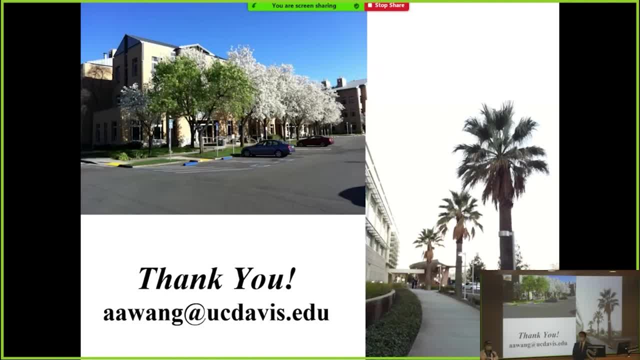 that have been associated with disease states. So I commonly see patients with Crohn's disease where they have just an inflammatory dysregulation, And so I'm wondering: is that part of what you're looking at, as well as the dysfunction? Yes, 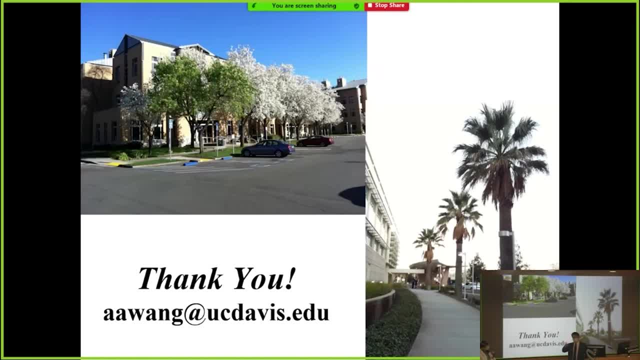 So, as you can imagine- I mean, as we discussed earlier- all the cells are able to make EVs And cells have different status and different stages that make different EVs, So you can actually distinguish, potentially you can distinguish EVs that are made by different populations of cells. 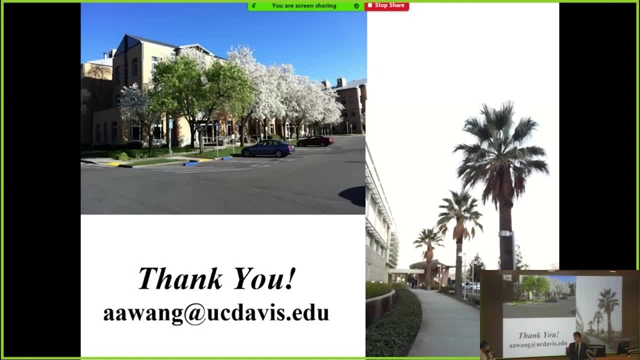 by looking at the surface marker expression, by looking at what's inside. So totally that's very doable, especially now with the nanotechnologies that we are trying to develop as a collaborator for biomedical engineering. Basically, we're trying to analyze single EVs. 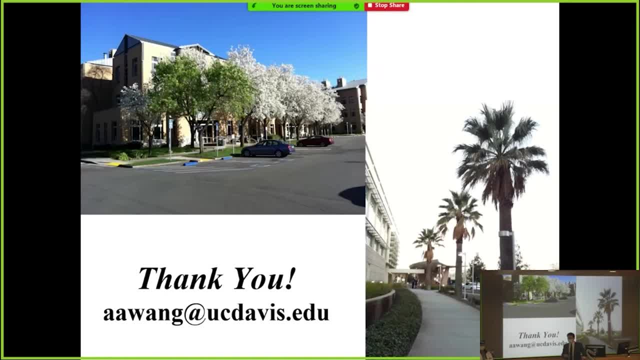 So we call it nanoteasers. Like Randy Carney is a professor from biomedical engineering trying to understand how to use those nanotechnologies to understand EV individually, one by one. analyze those And it's like you are doing single-cell sequencing. 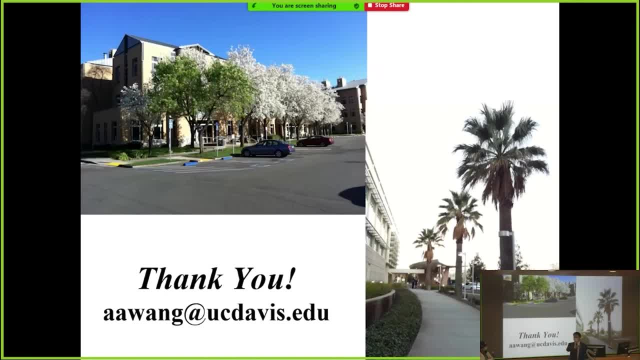 For example, nowadays, it's very powerful for you to understand the heterogeneity and also the population subpopulation of the cells in the body. We can also do the same for EVs, even though they're very small. Remember, they're only 100 nano. 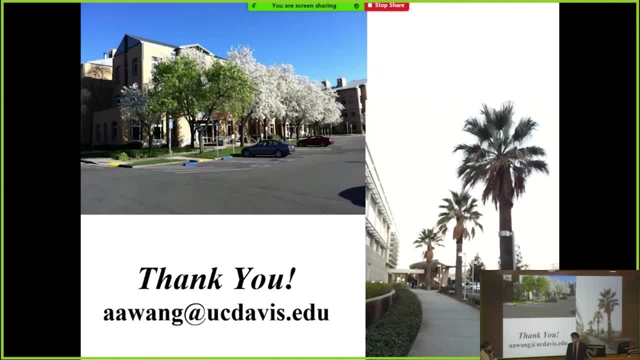 so very small, But it's doable And I think there's a huge potential for expanding that technology and doing that research as well, for biomarker discovery, for example. Back to the video world. Dr Sean Adams asks I should at some need to see this presentation. 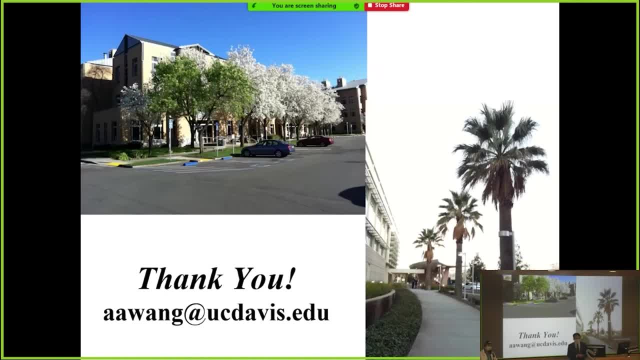 to learn more about the specifics of the studies you've been doing. Are folks developing coatings for tissues that are often the target of autoimmune attack, eg joint tissues? Could those spaces be coated with something that opposes inflammatory cell attachment? Yes, I think you know.